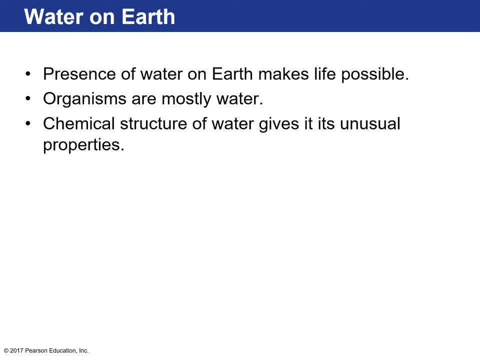 on Earth. You may know that water is really essential for sustaining all forms of life on our planet And, in fact, it's the primary component of all living organisms. About 65% of human makeup is water and plants are about 90%, So water is extremely important. 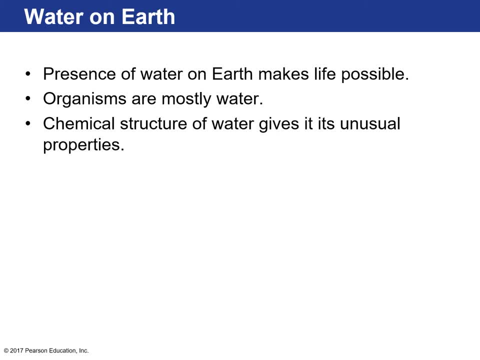 to all organisms on the planet. The chemical structure of water- H2O, two hydrogens and an oxygen- gives it really unusual properties and makes it very unique and also has specific properties. So water is important for our society as a whole. It is important to our 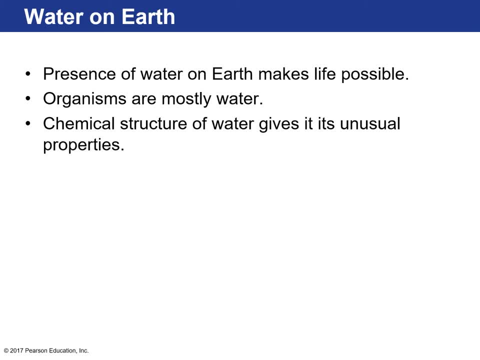 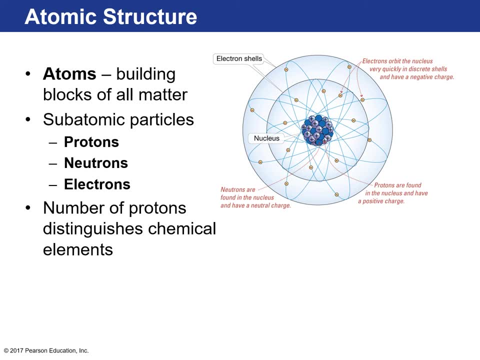 properties that actually help organisms on this planet survive. So if we go down to the atomic structure, just a little review. but atoms are building blocks of matter. They're made up of subatomic particles, protons, neutrons and electrons. 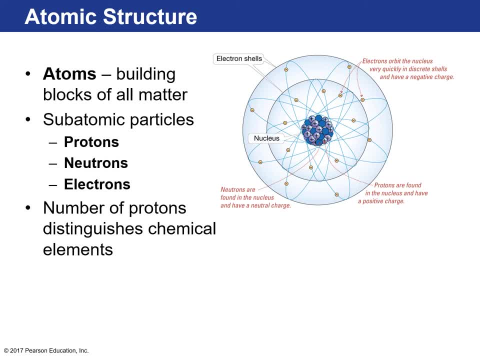 Protons are found in the nucleus and they're positively charged and they have mass. Neutrons have no charge, but they also have mass and they're also found in the nucleus. So this would be a depiction of an atom and this would be the. 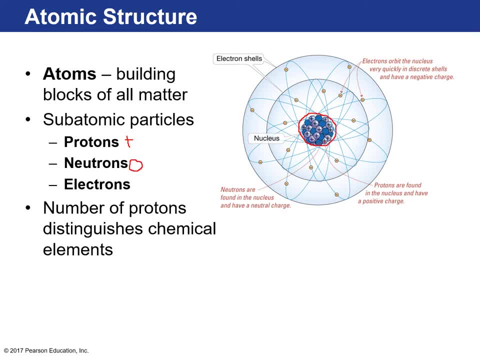 nucleus. here, Surrounding the nucleus are electrons and they have negligible mass and a negative charge, so they're kind of orbiting the nucleus in various electron shells surrounding the nucleus. So the number of protons, and that's always something that we find and that's something I like to be able to. 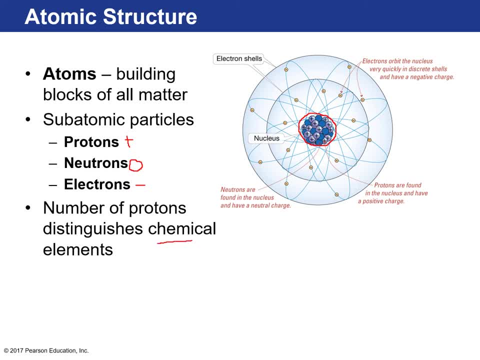 any atom distinguishes that chemical element. So for example, carbon has six protons and any atom that has six protons must be carbon. If you increase, if you add one proton to that, then you have a whole new element and that would. 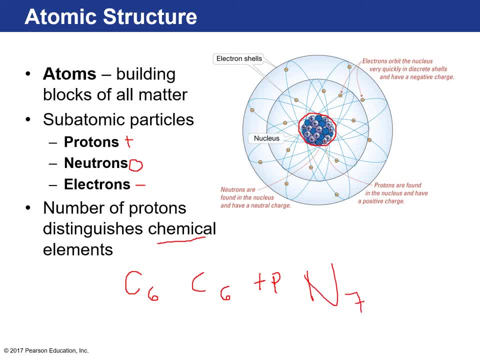 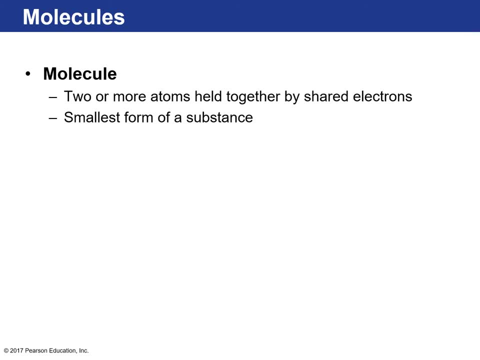 be nitrogen. Nitrogen has seven protons A molecule. on the other hand, a molecule is where you have two or more atoms that are held together or bonded together by shared electrons, and that's the smallest form of a substance. So when we look at, 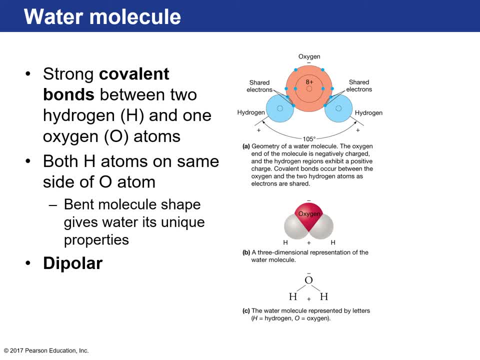 the water molecule, so H2O. we have a larger oxygen atom here in the center, and it has about six electrons in its outer shell. right. In order to achieve stability according to the valence rule, you have to add two electrons to it, and so what? 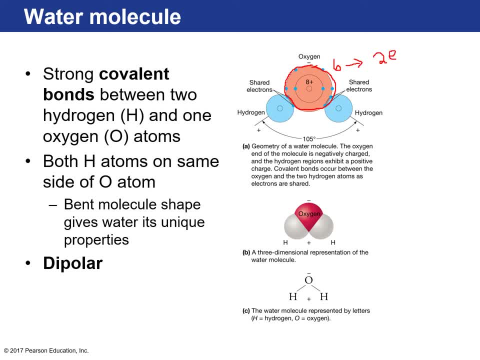 oxygen commonly does is bond with hydrogen. Hydrogen is just one proton and one electron, So hydrogen willingly shares its electron with oxygen and another hydrogen atom over here, and that's where you get the formula H2O. Oxygen is a very electronegative. 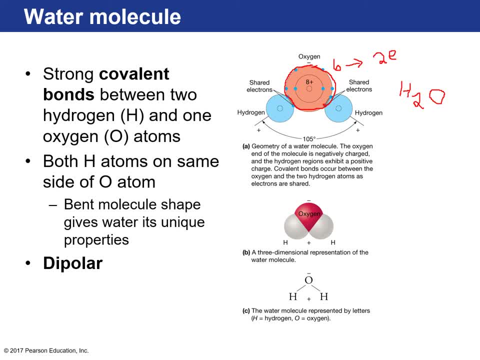 atom, meaning that because it's so close to having eight electrons in its outer shell, it kind of hogs the electrons and pulls them really closely. So what ends up happening is that the hydrogen atoms start to kind of move towards the bottom end of the oxygen molecule because of the high electronegativity from oxygen itself. 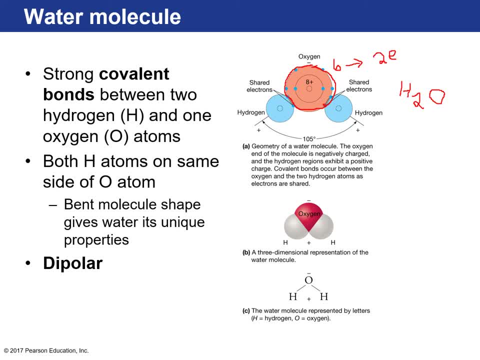 So it creates this kind of unique structure where the both hydrogen atoms are about a hundred and five degrees to one another. Normally what you would see with most molecules is that here would be hydrogen, here would be the oxygen and here would be the hydrogen, and it would be kind of 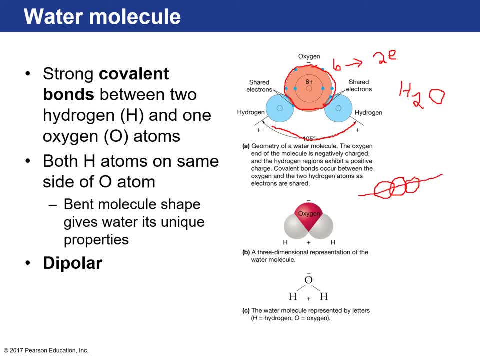 like a straight line with this bond. So what? what happens as a result of this bend is that it gives water very unique properties. One is that it's dipolar, and that means that one side of the molecule has kind of like an overall negative charge. 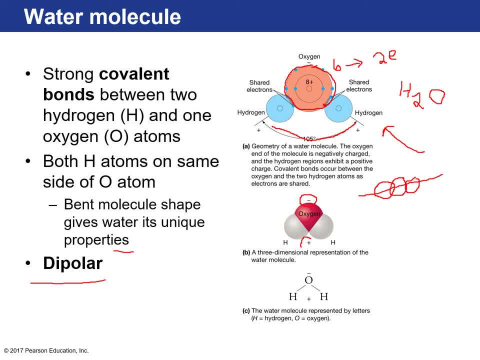 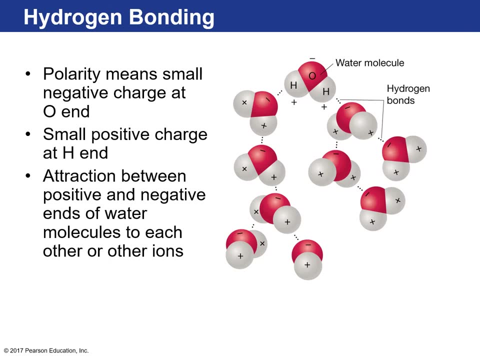 and one side has an overall positive charge, and that's shown in kind of these diagrams here written out. Okay, and so that polarity means that, like I said, there's positive and negative charges on either side of the molecule, and so what this does is this attracts other water. 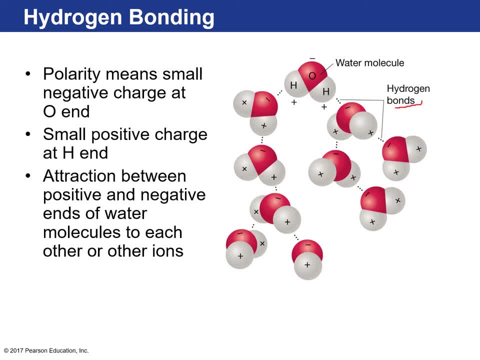 molecules and they end up bonding together in the form of hydrogen bonds. So there's an attraction in between molecules, individual molecules of water, and so the negative end of a water molecule is forms a hydrogen bond with the positive end of a different, of a different water molecule and 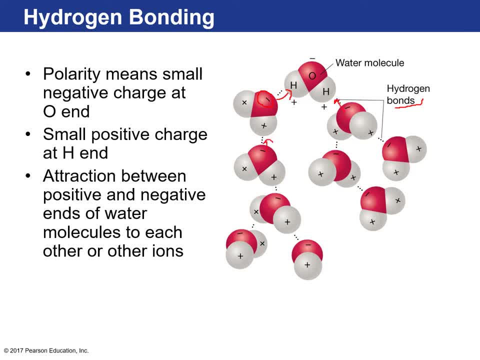 same over here and then so they start forming these links together. And that's how kind of water molecules bond to one another through these hydrogen bonds. Hydrogen bonds are weaker than the covalent bonds between the hydrogen and oxygen. so this bond right here, where they share the electrons between hydrogen and oxygen, it's called the covalent. 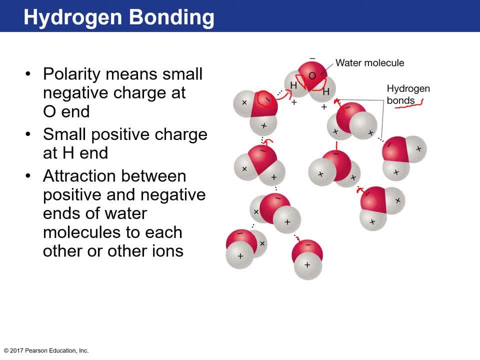 bond. Those are really strong bonds and they're very hard to break and you would have to put a lot of heat and energy into water to break those bonds. Hydrogen bonds with the covalent bonds have been able to do that both in solid and moh Newman. Uh uh uh. in the same way, left and right used as heterogeneous bonds, Uh uh uh. but here you can see we have here in the case of hydrogen, here you have uh, part of this we have aqui. uh, I got a little two- publishing Hi um the hydrogen Inflammation. 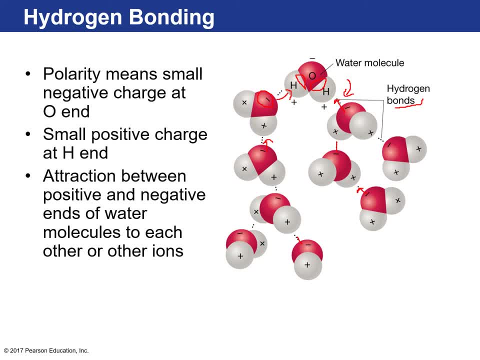 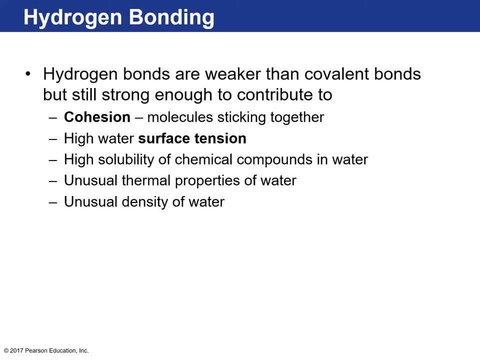 Hydrogen bonds are much weaker. It takes less energy to kind of disrupt the links between each water molecule. So the reason why we mention hydrogen bonding is because that accounts for or contributes to some of the properties of water. One is cohesion Molecules sticking together 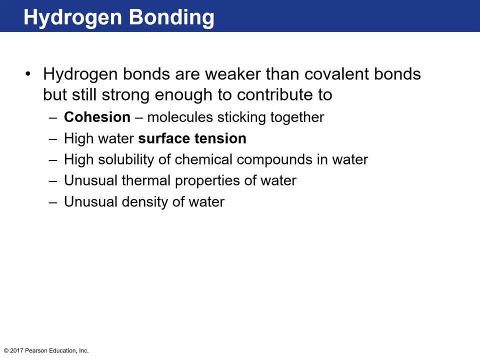 If you ever spill water like on a surface, maybe a kitchen countertop, you'll notice that a lot of times water kind of like bubbles together and links up together. Also, water has high surface tension, meaning that like one example is that, like you say, 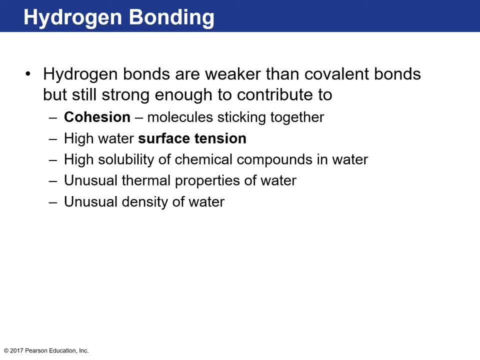 you pour a glass of water, you can fill up the glass completely and a meniscus will form. It's kind of like a concave shape Above the rim of the cup, So like water can be piled into the cup above the actual rim. 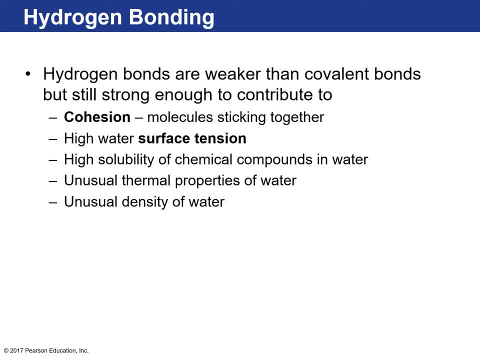 And that's because of that surface tension and cohesion, with water molecules kind of sticking together. Also, water is, you know, you might not think of it, but it is kind of sticky. After you get out of a shower you have water. 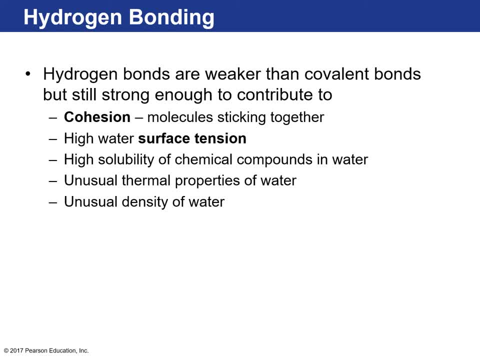 Water isn't just repel off of your body, right, It is kind of like sticks to your skin And that's why you have to towel. Another interesting property of water is that it has high solubility of chemical compounds, meaning that if you put solids into water, it can dissolve some solids. 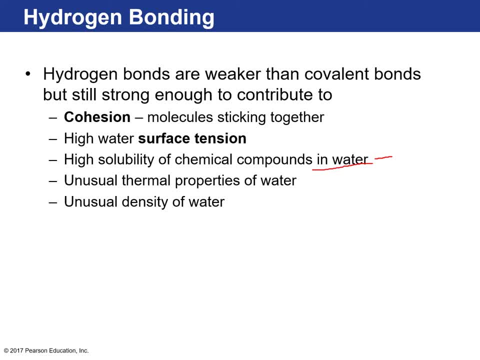 And so, and it can keep a lot of dissolved solids in suspension in the water It also has. water also has very unusual thermal properties, which are very important In terms of how heat is distributed in earth and how it affects our climate. 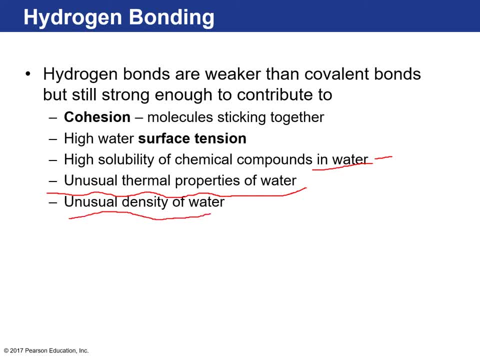 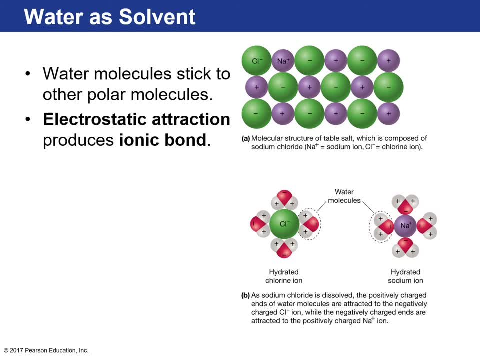 And then also water has an unusual density or change in density when it goes through phase changes. Okay, So water is a solvent. Let's take a salt, for example, that is NaCl, So you have a sodium ion here and a chlorine ion, ion. 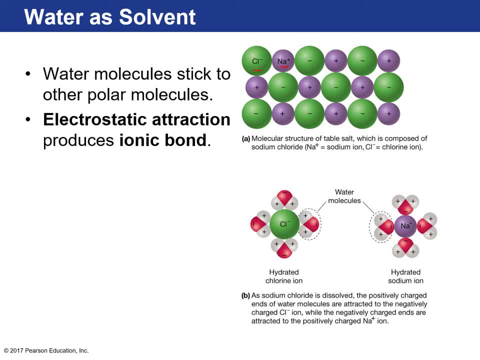 They're bonded together by electrostatic attraction. What's that? They're ionic bonds. And so if you have like a glass of fresh water and you start putting salt in it and you start mixing the water and salt, the water molecules themselves, the positive ends will start ripping. 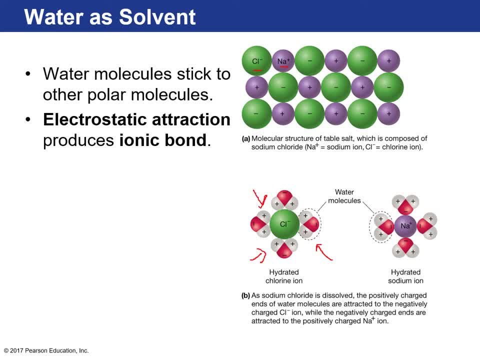 the chlorine atoms from the structure. Okay, So they'll remove the negative chlorine from the salt and then the other ends of the water molecules will pull the positive cation from the structure, And essentially that's what dissolving is. It's just it rips those ionic bonds apart. 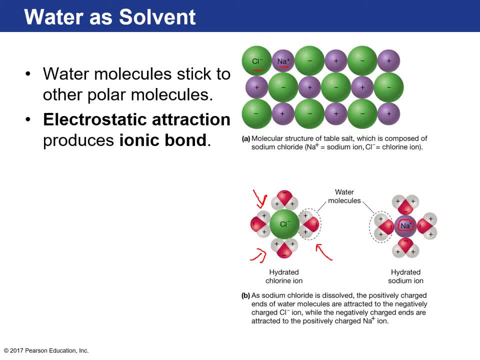 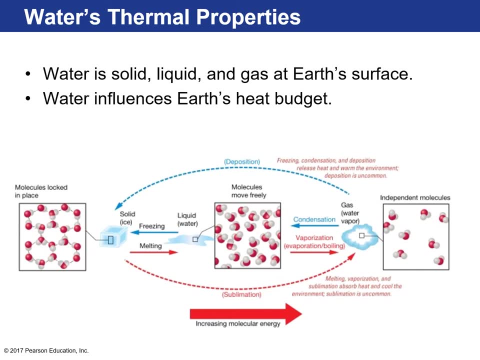 And then those ions kind of remain with the water in suspension. All right, Water also has very unique thermal properties. On the earth's surface you can find water as a solid liquid and gas, especially in the atmosphere, And that influences the heat that travels ethically. 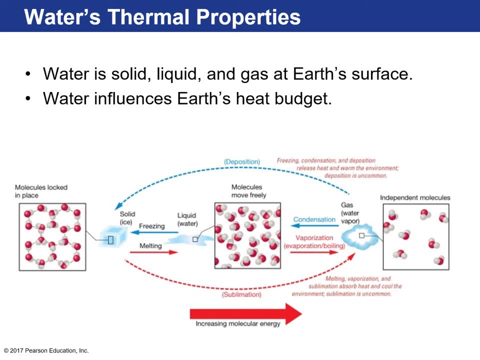 Okay, Throughout the earth. And the reason is because water has a unique property of distributing heat as it goes through phase changes. So if you look at solid water where the molecules have formed a crystal structure, you can see that here all the individual molecules have kind of bonded together into a solid 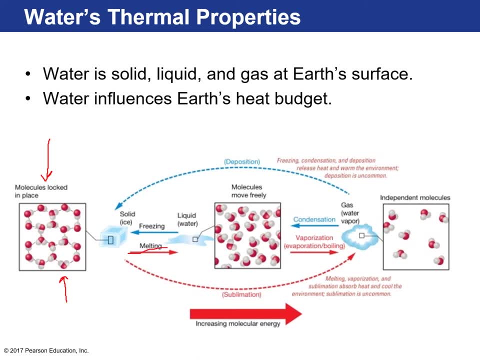 When a solid ice melts into a liquid. so this is a liquid. over here, where the molecules have the ability to move freely, they'll still form those hydrogen bonds as a liquid. And when a liquid turns to gas, we call that either evaporation or boiling. what happens? 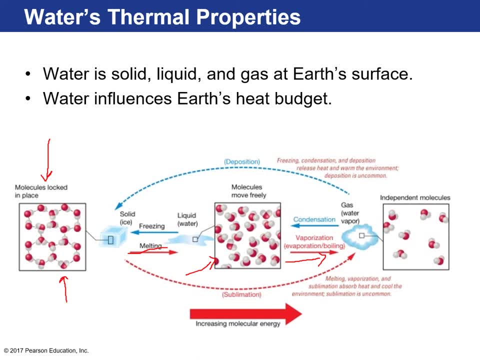 Those three processes- melting, vaporization or evaporation, or sublimation- which is going from a solid all the way to a gas which is less common. Okay, Okay, Okay. So the solid is in the air, So this is the gas. 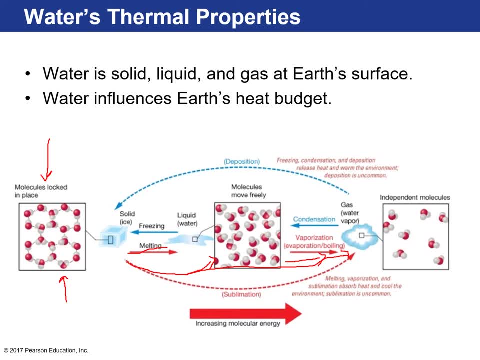 It controls the environment around them, So it absorbs heat from the environment, So it takes heat from the environment every time it goes through one of these phase changes, If you go in the other direction from gas. so this is independent molecules, water molecules. 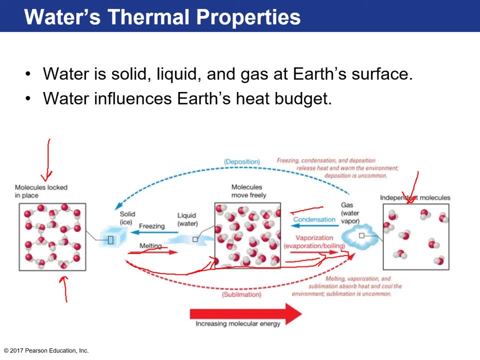 in the air and that condenses to form a liquid. or you have a liquid condensing even further and freezing to form a solid. freezing, condensation and deposition. that all leads to a release of heat into the environment. so heat is actually being released into the environment. so you can see as, as water moves. 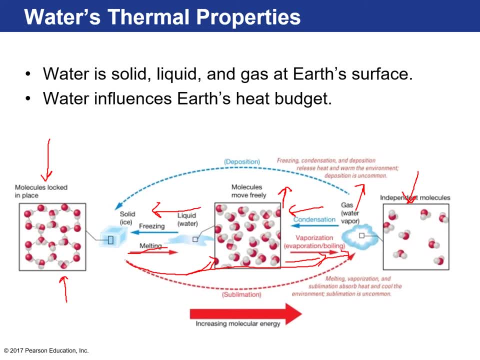 through, let's say in ocean currents or water vapor in atmospheric currents, into different regions of the earth. it will transfer heat. it'll absorb heat from areas, carry it around and then release it, so it kind of moves heat depending on which direction or phase change is occurring. 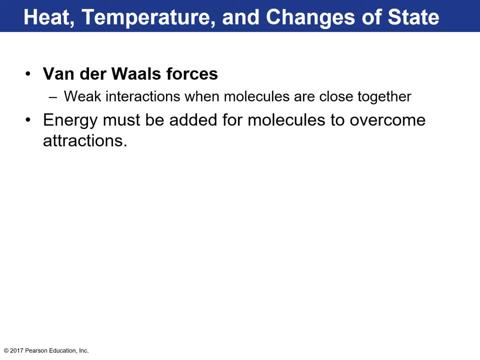 van der waals forces are kind of these forces that hold individual molecules together. they're relatively weak interactions and it exists between electrically neutral molecules because of kind of an uneven distribution of charge. okay, so in order to kind of uh, have water go through phase changes like gas, 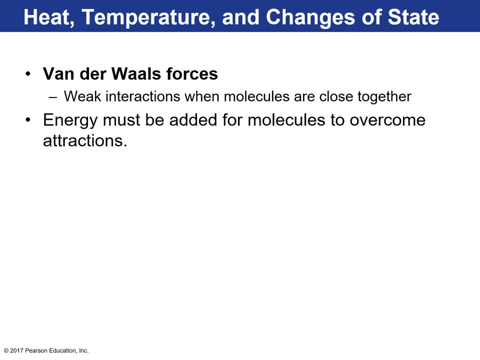 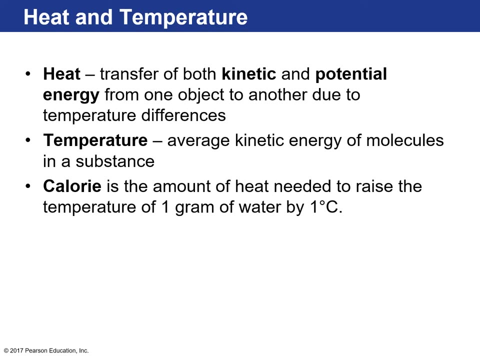 to liquid, to freezing or the other way around. energy must be added to those molecules to overcome those van der waals forces, as well as the hydrogen bonding between each molecule. so let's take a step back to to understand the phase changes of water and how heat is distributed. 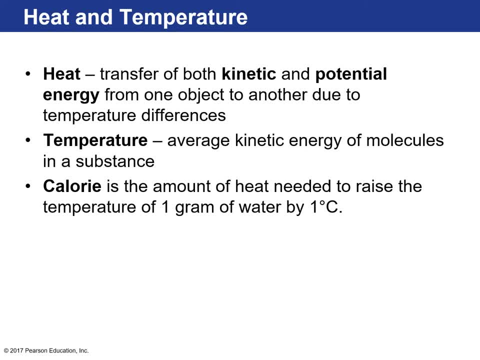 uh, throughout those changes by understanding heat and temperature. heat is a transfer of both kinetic and potential energy from one object to another due to temperature differences. okay, so, um, think of something that's really hot, maybe a stove top, and you put something cold on top of it. heat is going to transfer from the hot stove top to the 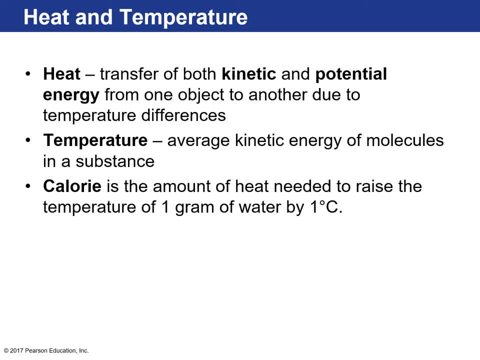 or skillet or whatever it is, and heat is something that you can kind of, you can measure in an object something that it can contain, okay, temperature, that is the measurement of the average kinetic energy of molecules in a substance. so it's kind of like a moment in time when you're finding out how, how kinetic or 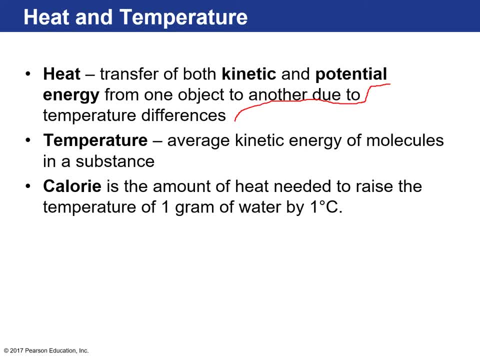 how much kinetic energy is in an object, right, how hot it is, the hotter an object is, and we measure that in Fahrenheit and centigrade. but if something has really high temperature, that means it has really high kinetic energy and it's really hot. okay. but that's temporary, right. it can cool down or it can heat up. 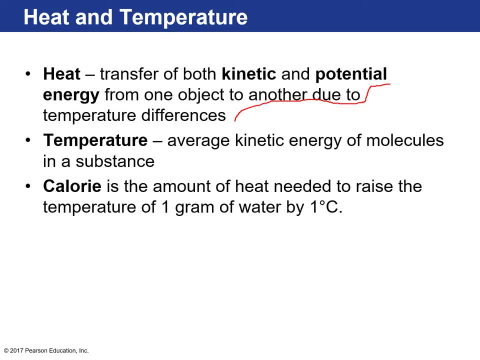 and in some cases so that's kind of like a measurement of a moment in time. okay, so like to understand the difference between heat and temperature. let's take like, say, you fill a bathtub with really hot water and you're gonna take a bath, and then you 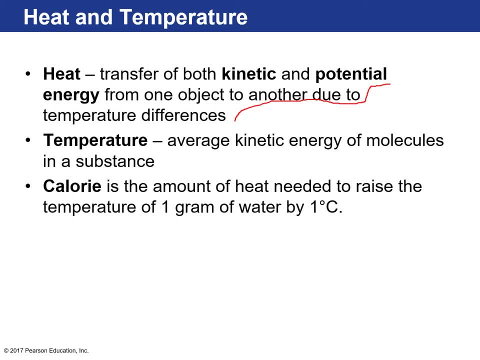 also have a candle. okay, this got really romantic, but you have a candle and you've got a flame on that candle. now, if you measure the temperature of the flame in that candle and the temperature of the bath of water, the temperature of the candle and the temperature of the bath of water and the temperature of the 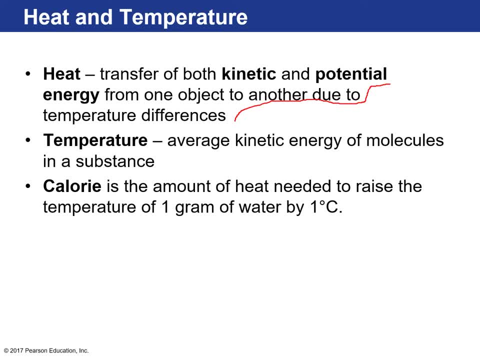 candle flame will be much higher, meaning that the average kinetic energy of the molecules that are involved in that combustion is higher than the than the temperature or the average kinetic energy of the water in the tub. but You can. the water in the bathtub holds more heat energy like it, because there's more. 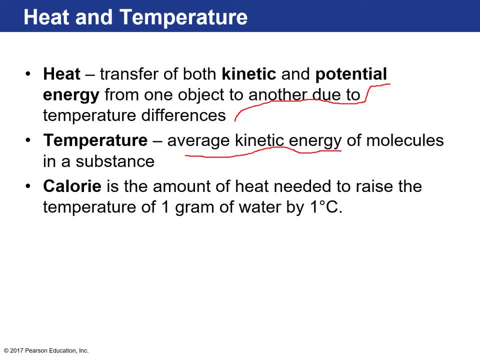 water, a bigger volume, there is more heat being stored in the bathtub. a stops all the heat. you are samping, then there's heat in that kind of flame. so even though the flame is hotter, has higher temperature, there's more heat in the bathtub. okay, and then a calorie is. 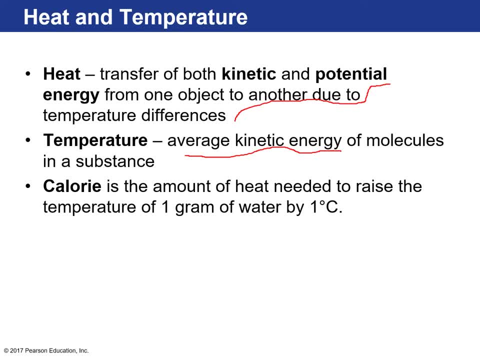 the amount of heat that's needed to raise the temperature of one gram of water by one degree Celsius. so say you wanted to increase the temperature of your, your bath, your bath water. you'd have to add heat to it, and then you'd have to have calories and calories of heat to increase its temperature. so 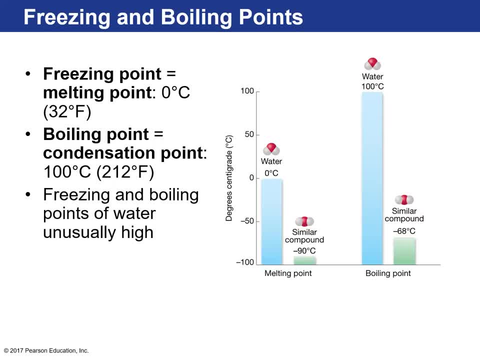 basically adding heat to the water. so if you add enough heat energy to any solid, it will melt into a liquid, and if you continue to add heat to a liquid, it will evaporate or vaporize into a gas. okay, this is true of all substances. right, water has unusual. 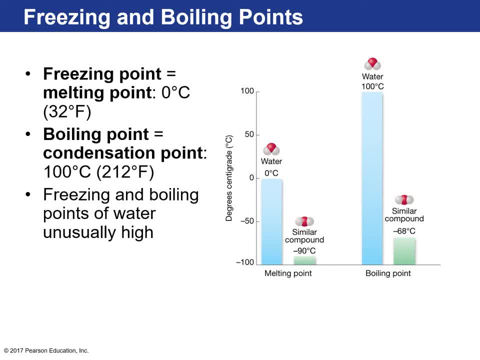 freezing and boiling points. the freezing and boiling points of water are high compared to similar chemical substances. okay, the freezing point- or melting point, depending on the direction you're going in- is zero degrees Celsius. okay, the boiling point is about a hundred degrees centigrade. okay, those. 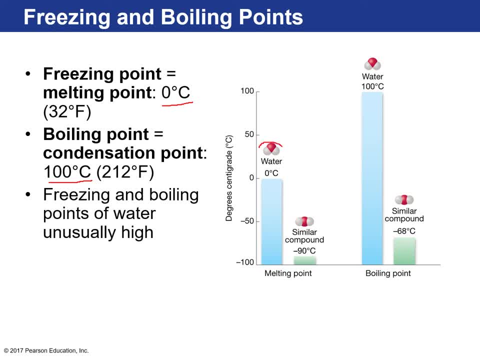 those are unusually high. and if you look at water, this is compound. remember, has that bent dipolar type property. a similar compound, without that, would have a melting point of negative 90 degrees centigrade, okay, and have a boiling point of negative 68 degrees Fahrenheit. 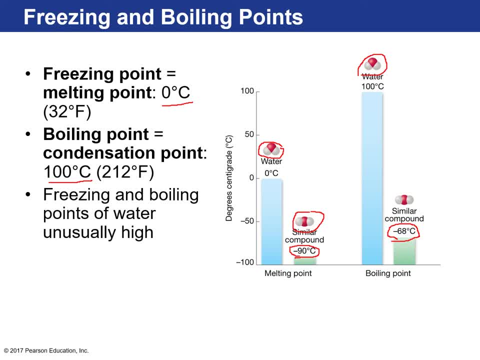 all right, so that that is unusual. there's a big difference between water and it takes a lot of heat that you must add to water in order to make it boil. other substances you don't have to a lot add a lot of heat for it to boil away, or 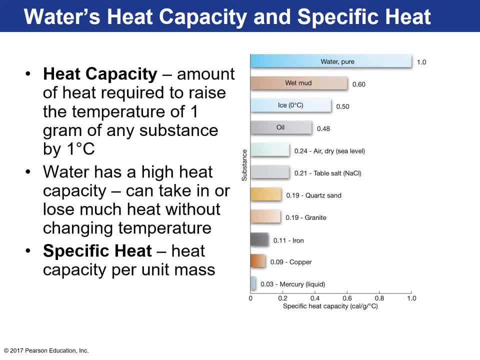 you know, evaporate away, and that's important, because what that means is water can hold a lot of heat. I'm sure you've had this experience where you're like, all right, I want to boil some pasta for, let's say, mac and cheese, or you're making a you know some sort of pasta meal, and then you get all this. 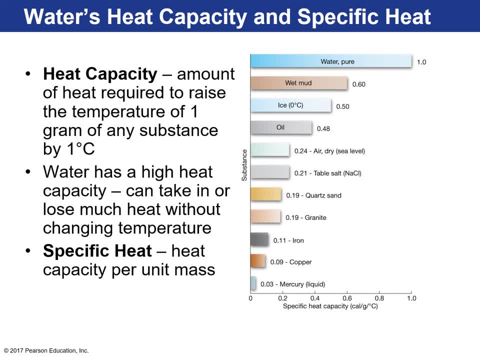 water, put it on the stovetop and you're waiting for it to boil. it takes forever. sometimes that happens especially if you're trying to bring water to boil that's at room temperature. it can take a long time, and the reason is is because water has high heat capacity. okay, heat capacity is the amount of heat required. 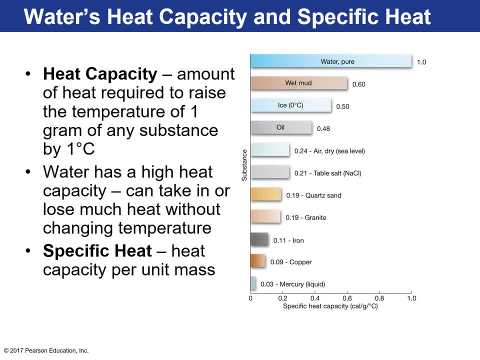 to raise the temperature of a substance one gram by one degree centigrade. okay, so water has high heat capacity, which means it can take in a lot of heat or lose much heat without a drastic change in temperature, and that's critical. okay, so think about that. here's pure water with high heat capacity. okay, things that. 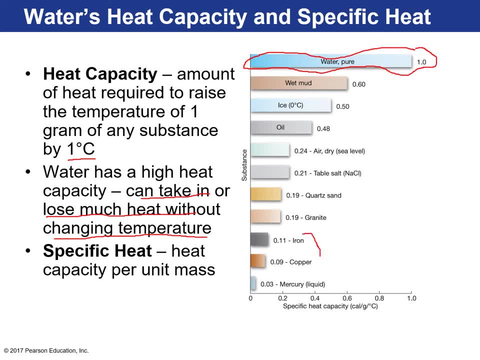 we don't want to have high heat capacity- iron and copper, for example- I wouldn't say we don't want it, but I would say we don't want it because we don't want to have high heat capacity, and so because of that, we use them as pots and pans. why? 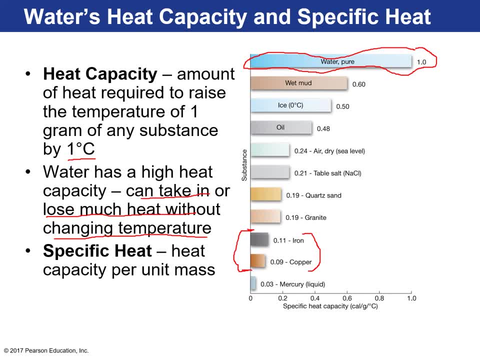 because they don't have very high heat capacity, meaning that as soon as you apply some heat to those substances, the heat moves through them and heats it up really quickly. so it will cook your food really fast, because the heat is gonna transfer through the copper and into your food, right. so that's why we use 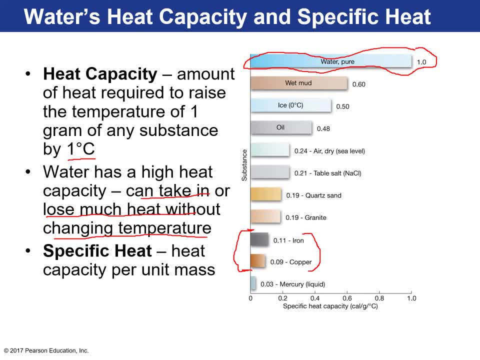 them as pots and pans because that's such low heat capacity. another example of this would be like, say, you go to the beach right a lot of times, especially in the summertime. if the Sun is out, the Sun will be hitting the sand and the sand gets really, really hot. so you have to kind of like quickly. 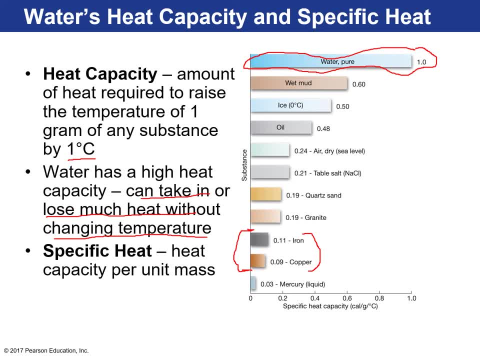 shuffle, shuffle your way to the water, where it's much cooler. well, yeah, if you look at quartz sand, which makes up a lot of beach sand, it has a much lower heat capacity, meaning that the surface of the sand is gonna get really hot and potentially burn the bottom of your water. so that's why we use them as pots and pans. 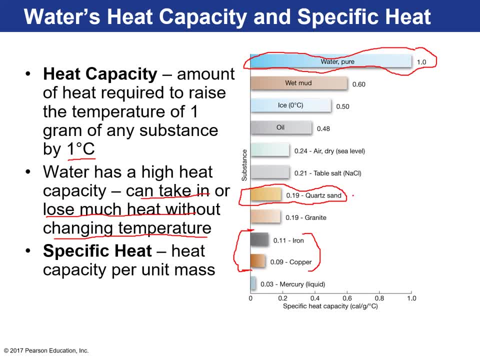 right- whereas the water temperature in the ocean- fortunately in these hot Florida summers it won't heat up that surface water so drastically, so ocean water kind of remains mild, let's say it doesn't heat up so quickly and doesn't cool down so fast, and that's because of the heat capacity of water. we also refer 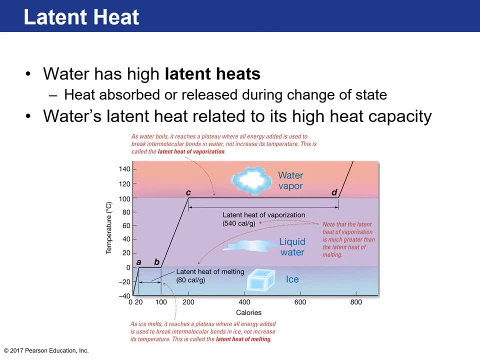 to this as specific heat. then there is latent heat. water has high latent heat. what latent heat essentially means is hidden, so to speak. okay, so water has the ability to absorb a lot of heat when heat is being added to it. okay, and when there's a major 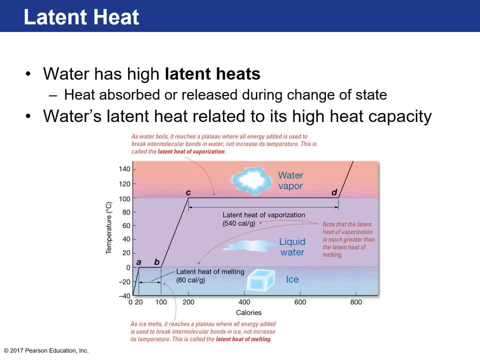 change of state, meaning like going from a solid to liquid or to a vapor. there's a lot of heat that's released during that change of state. okay, and that is related to its high heat capacity. right, and it makes sense, because what will happen is, if you add heat to water, the temperature won't change that quickly. right, it takes. 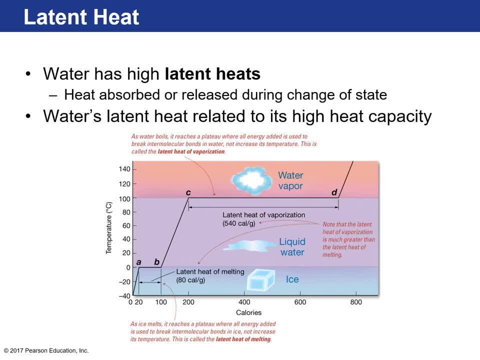 a lot of heat to change that temperature. and specifically when you're going through a phase change- like say you're going from ice to liquid water, as you add more and more heat the temperature of that mix will not change. so if we look at this diagram here, you can see at the bottom we have calories and heat. 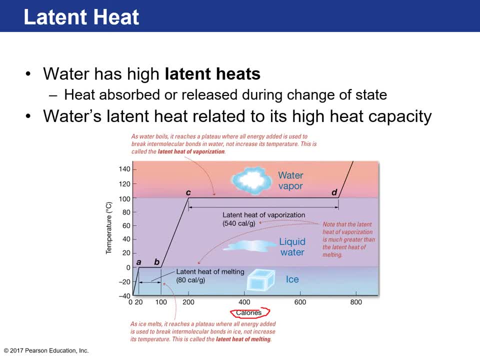 okay, and then here we have temperature, all right, and then a, B, C and D are different kind of junction points where there's a phase change or a drastic change in either the temperature or a phase change in the in the water. okay, so if we start over here with ice, right, we're really low temperatures. and if we 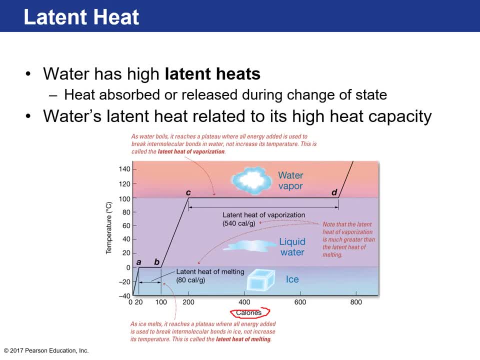 start adding heat to that ice, the ice is going to absorb that heat and its temperature is going to start to rise. okay, until it hits point A. okay, Point A is when the ice starts melting at zero degrees centigrade. all right, And so what's interesting is it's going through. water's going through that. 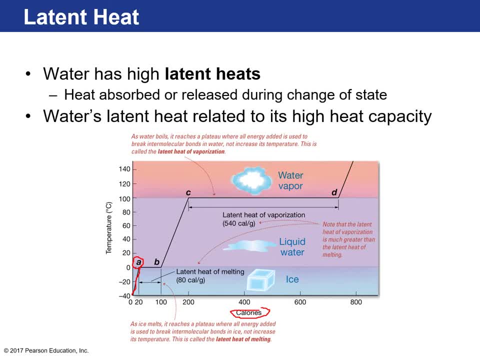 phase change going from ice to liquid water, And when that's occurring, you're adding more and more heat, right? So if you're moving along this direction, right, you're adding more and more calories to that ice and water mix, but the temperature remains at zero degrees centigrade. 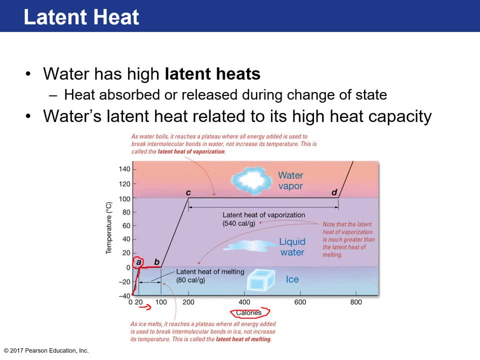 And that's what latent heat means, Because that's, you know, what perplexed a lot of people doing these measurements is when you're melting ice and you're taking its temperature. the solid ice block at zero degrees centigrade is the same temperature as a mix of ice and water. 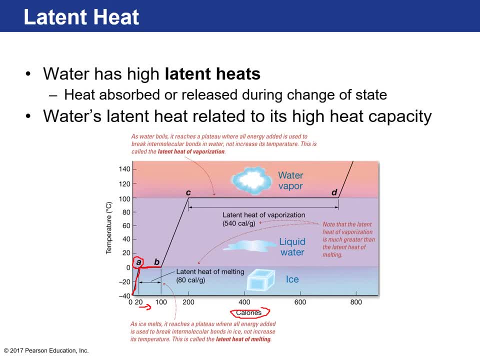 together zero degrees centigrade, And the temperature of the ice block is the same temperature as the temperature of the liquid water. So when you're melting ice and you're taking its temperature, the temperature of that mix will only go up until all the ice has completely melted, And that's point. 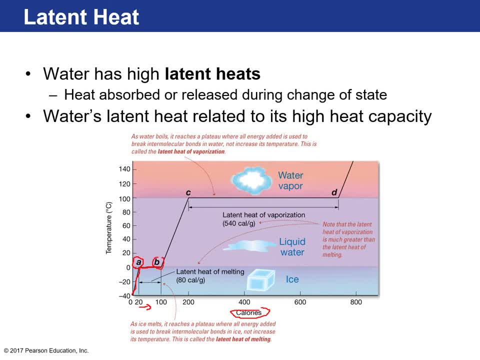 B right here. okay, So as ice melts it reaches that plateau and all the energy that's added is used to break up the kind of intermolecular bonds in ice and it does not increase the temperature. So that's called the latent heat of melting. all right, And that's approximately. 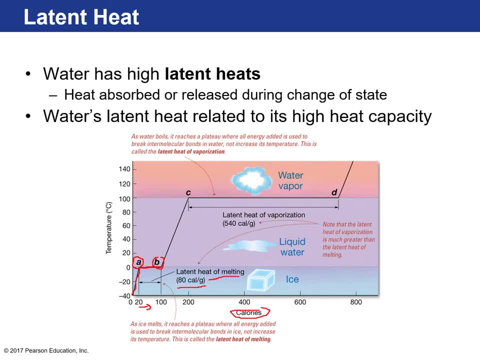 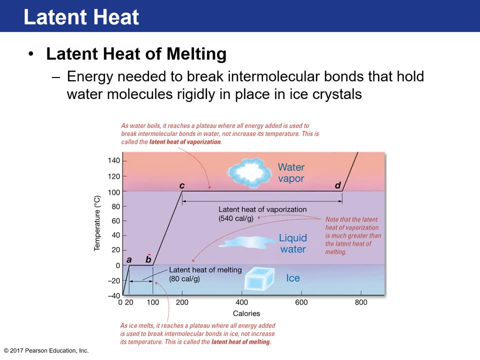 80 calories per gram. Okay, if we continue from spot B, and now we're at liquid water just above zero degrees centigrade, and we continue to add heat. so we're moving in this direction, continuing to add heat- what you notice is the temperature starts to rise. So if you have a liquid and you 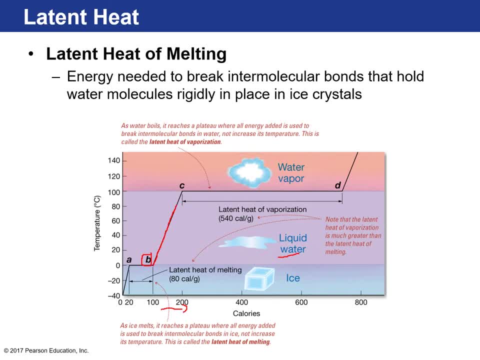 continually increase or add heat to it, the temperature will rise until it hits the next plateau at C, And that next plateau is the water begins to boil. okay, And you're going from liquid water to water vapor. okay. And when that occurs, then you start have to kind of not only break the 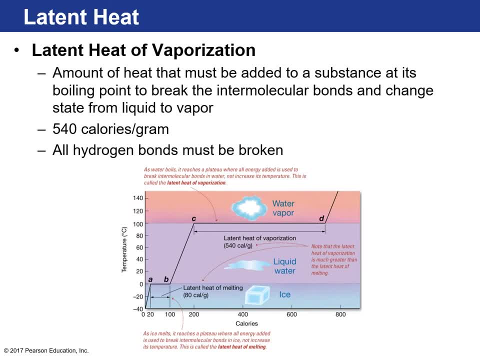 intermolecular bonds. okay, And that's referred to the latent heat of vaporization. All right, that's the amount of heat that must be added to a substance at its boiling point to break the intermolecular bonds and change the water from liquid to vapor, And it's approximately 540. 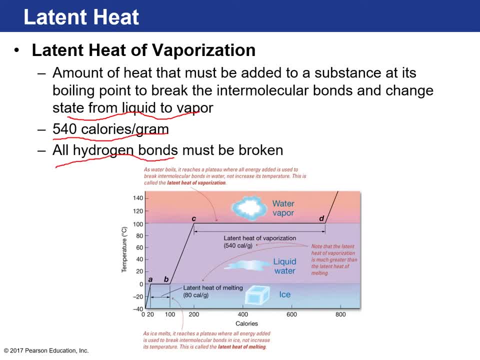 calories per grams And every single hydrogen bond in between every water molecule must be broken. okay, So that's here. So say you have boiling water, right. You can continue to add more and more heat, right? More and more calories as you travel in this. 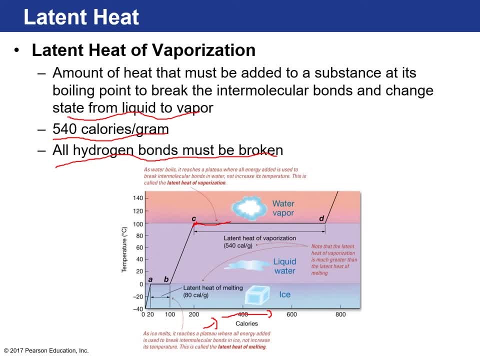 direction, but the temperature of that boiling water will remain 100 degrees Celsius. It'll do that until- and this is assuming that you have a closed system- so all the water vapor is being trapped. Let's say you have like a top to that boiling water and all the gas molecules are. 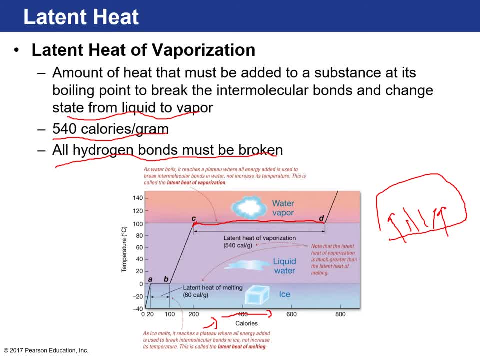 being trapped. okay, So until you've boiled all the liquid water away and then you've added all that water is in its gas phase, and water vapor only does the temperature increases once you get to point D, right here, And that's when, here you see, that temperature starts going. 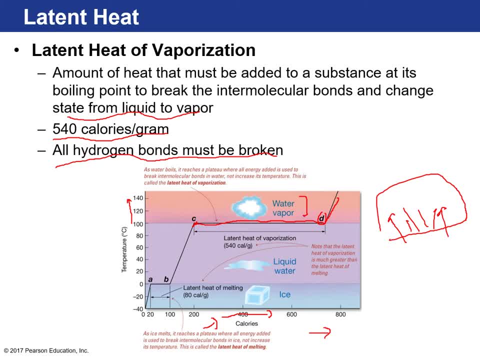 above 100 degrees Celsius, And that's because all the water is gone. And we call that the latent heat of vaporization, the hidden heat of vaporization, because this is the heat that's being added without seeing a drastic temperature change, as you're going from liquid to water vapor. 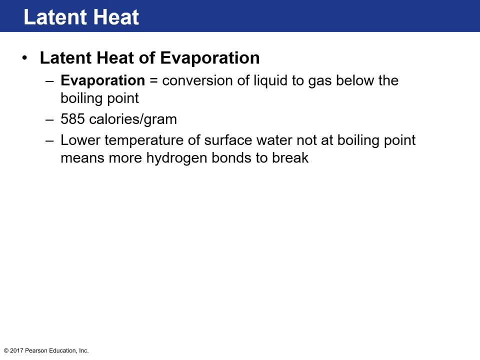 Latent heat of evaporation essentially is the conversion of a liquid to gas below the boiling point of water. So ocean temperatures rarely hit 100 degrees centigrade but evaporation still does occur in the oceans. So what happens here with evaporation, say in the oceans, is an 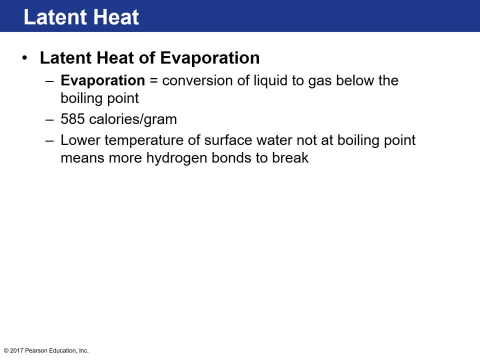 individual water molecule will. in order to break free from the surrounding ocean water and enter into the atmosphere as a gas, it must capture the heat energy from its surrounding neighboring water molecules. So the molecules left behind will have given up heat, so that that one molecule can. 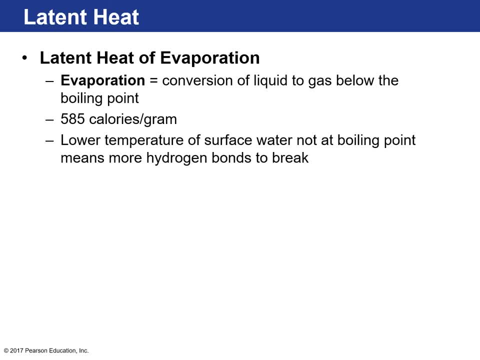 evaporate And that explains kind of what's going on in the atmosphere. And that's what's going on in the atmosphere And that explains kind of what's going on in the atmosphere. And that explains kind of what's going on in the atmosphere And that explains kind of the kind of cooling effect of evaporation right. 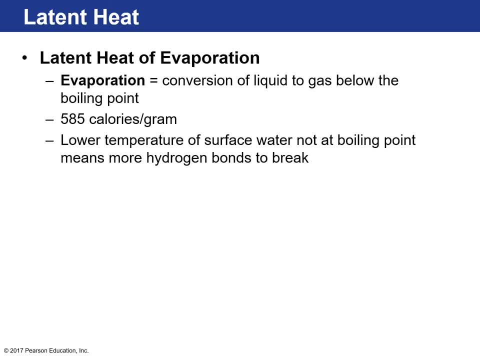 Like whenever you work out and you start sweating, right, you have beads of sweat surrounding on your skin and then that evaporates away. And when it evaporates away, it absorbs heat from your body and into the atmosphere and that's why you cool down, That's why we sweat when, whenever we do. 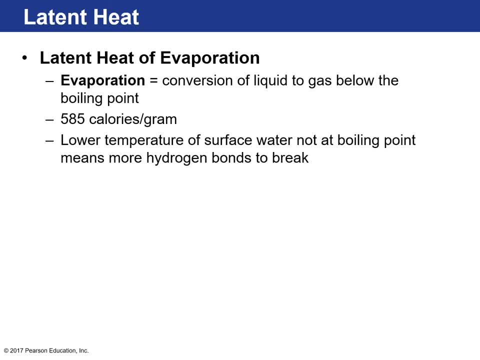 exercise. It's the body's response to our increased temperature and it wants to regulate and cool ourselves down, And that latent heat of evaporation is about 585 calories per gram. Okay, Then there's the latent heat of condensation, So we're going in a different direction here. 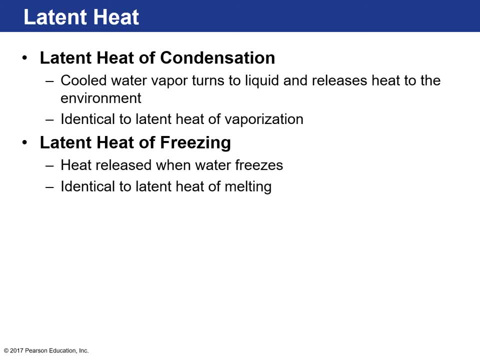 Cooled water vapor turns to liquid and then releases heat into the environment. So this is the same as the latent heat of vaporization, Just going in a different direction, going from a gas to a liquid. So this is the same as the latent heat of vaporization, Just going in a different direction, going from a gas to a liquid. 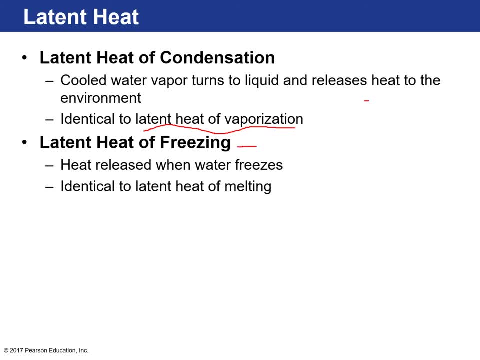 then finally, latent heat of freezing. so heat is released when water freezes. so when you have, you go from a liquid water to a solid. as it freezes and becomes a solid, heat is actually released, and that is equivalent to the latent heat of melting. so here we go. these are the different hydrogen bonds in all three. 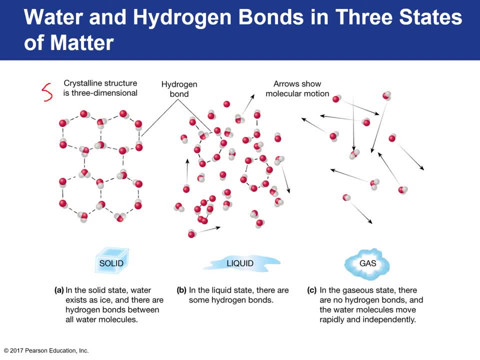 states of matter for water. this is the solid three-dimensional crystalline structure bonds between each one of the water molecules. when you go from a solid to a liquid, there are some hydrogen bonds, not not every molecule. some are free, completely free-moving. some are bonded together and then, when you go to 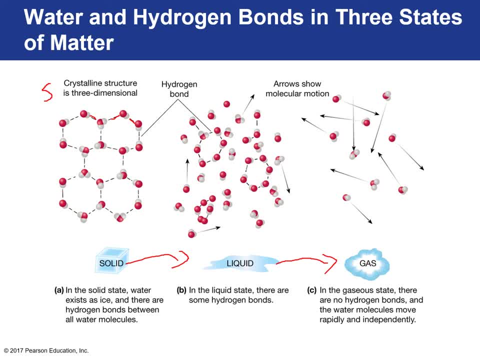 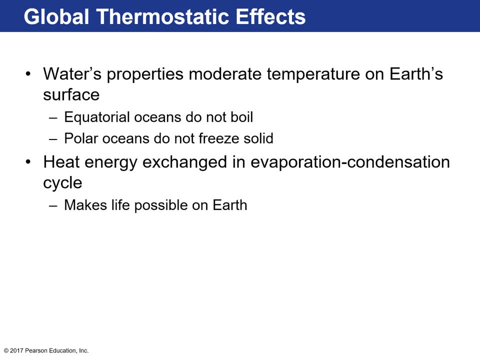 a gaseous state and, in terms of water, all molecules are free to move wherever they want. so what does this happen? what does this have an effect on the thermostatic effects of the water and how does it affect the temperature? and what are the effects on Earth? well, it helps moderate the Earth's surface. 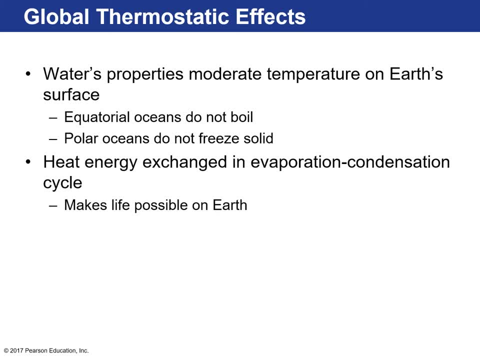 temperatures. when you're at the equator, the ocean water doesn't just boil off and boil away, and when you're at the poles of our Earth, the oceans don't freeze solid okay. so heat energy is exchanged, as water kind of moves through these different states as it evaporates or condenses it. 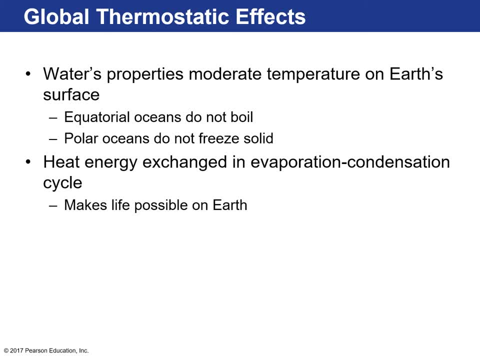 helps kind of transfer heat to different environments, and that's what really makes life possible on Earth. for example, in like really cold areas, let's say the air temperature drops down below zero degrees centigrade, that would freeze water right. the water is unique in the fact that ice floats, so when it 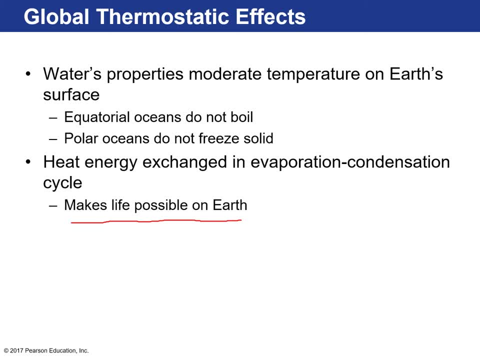 turns into a solid. it's less dense than the surrounding liquid, so a skin. so if you look at a lake right and it's below, freezing, the outer or the top layer of the lake will freeze solid kind of above the water and that helps insulate the temperature below that kind of outer frozen. 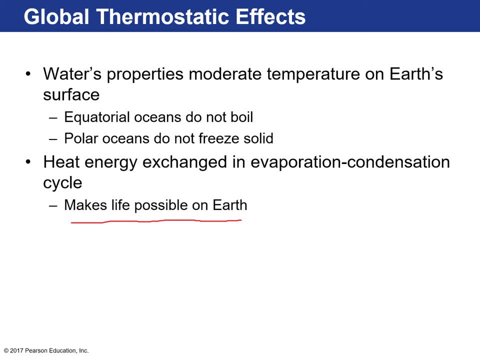 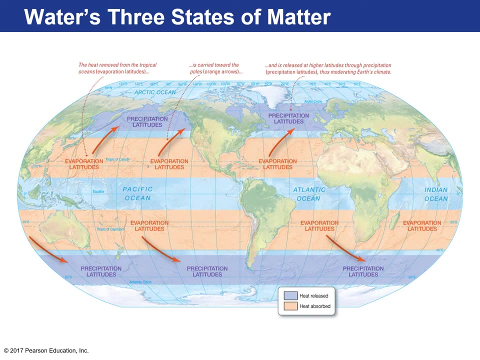 layer, and that keeps the fish underneath warmer, essentially because they're insulated with that layer of ice on top. so water has very unique effects, and so when we look at our globe, we have latitudes where there's a lot of evaporation. we call those evaporation latitudes. okay, this is. 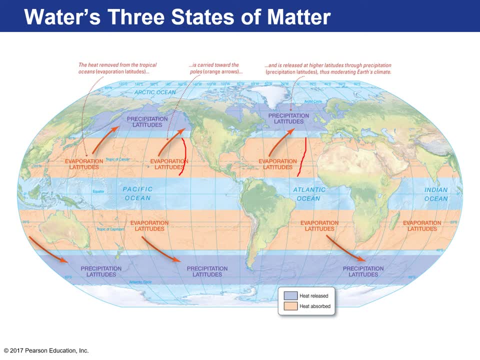 where evaporation exceeds precipitation and a lot of heat is removed from the oceans here and travels through air circulation and brings a lot of heat to polar latitudes right. so that helps distribute heat to colder regions and essentially it cools down these latitudes which are really hot and 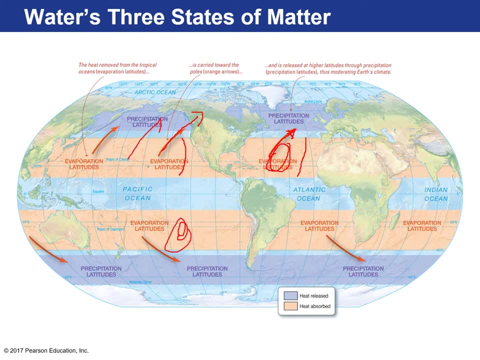 these latitudes are really hot and then helps transfer heat to cooler regions, And so that's why these lower latitudes don't boil away. and then these higher latitudes don't freeze completely, because heat is being transferred from warmer areas to cooler areas. 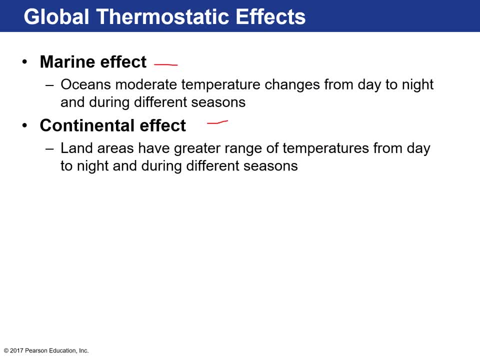 And so that leads to really cool effects like the marine effect. So if you're surrounded by an ocean, that helps moderate the temperature from day to night, meaning that there's less of a range in temperatures. It kind of moderates, it makes it milder. The continental effect. 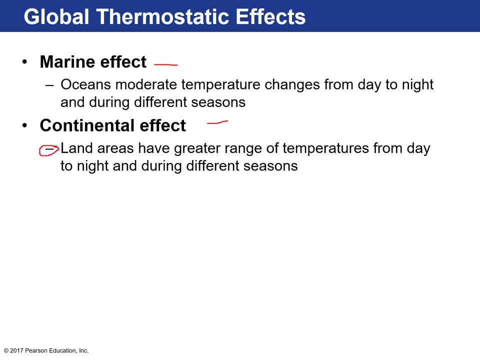 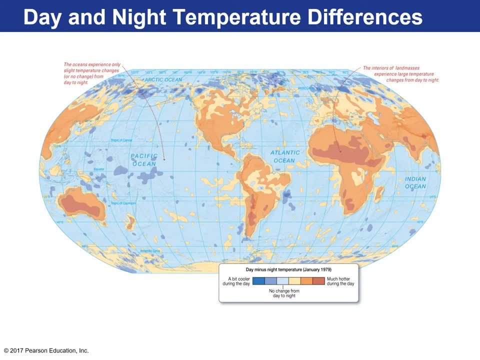 because land has such low specific heat, it has a greater range of temperatures from day to night in different seasons. So what that essentially means is like say: if you're in the middle of the continent, you're in the middle of the continent and you're in the middle of the. 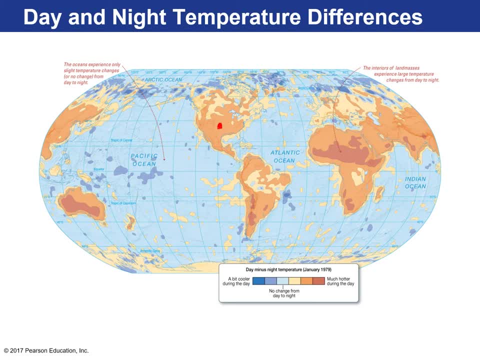 continent, and you're in the middle of the continent and you're in the middle of the continent. here in the United States, say the Midwest, it's much hotter during the day than at nighttime, So the days get really hot and then at night it cools down dramatically. But if you're 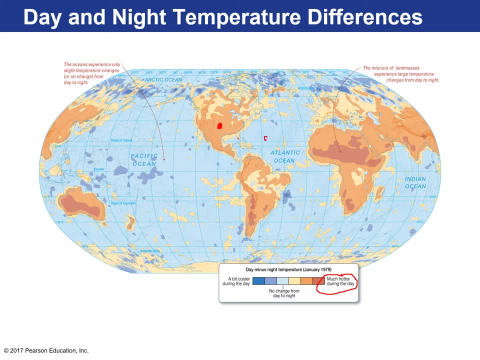 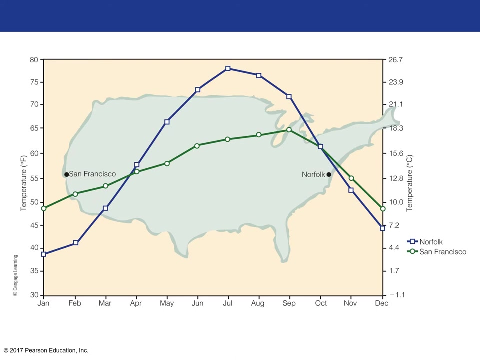 in Florida, like we are, or if you were out in the ocean, those differences in daily ranges in temperature are minimized, And the reason is because water can absorb a lot of heat And so it doesn't affect the air temperature above the water. Let's compare two cities. Okay, we've got. 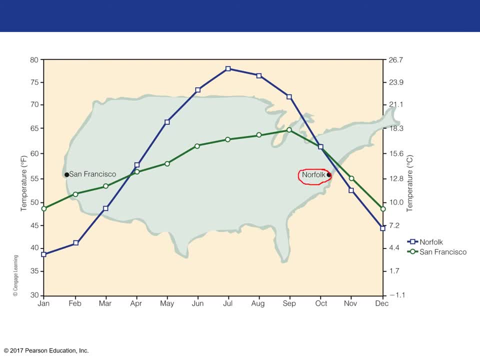 Norfolk Virginia on the east coast and we have San Francisco here. Okay, so the prevailing winds are in this direction. Okay, So what happens is San Francisco typically gets air masses that have been sitting over the ocean and move in through San Francisco In Norfolk Virginia. 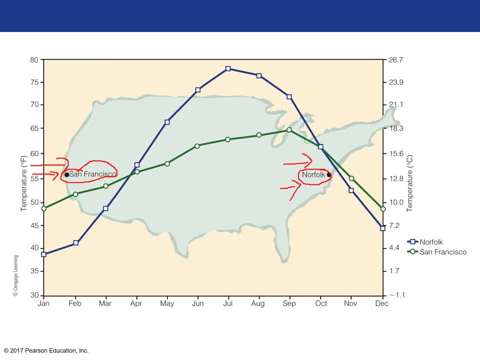 again, they're at the same latitude, so they'd be receiving the same amount of sunlight during throughout the year. On the x-axis, here you see all the months of the year, January to December, And on the y-axis temperature in Celsius or Fahrenheit. Okay, So because San 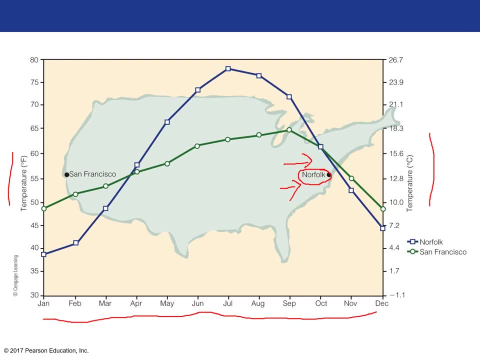 Francisco is over the ocean. its temperature is milder, meaning that during the winter months, January and February, it's actually warmer than Virginia, And during the summer months, April to September, it's cooler. right In Virginia, during the winter months it's really cold. 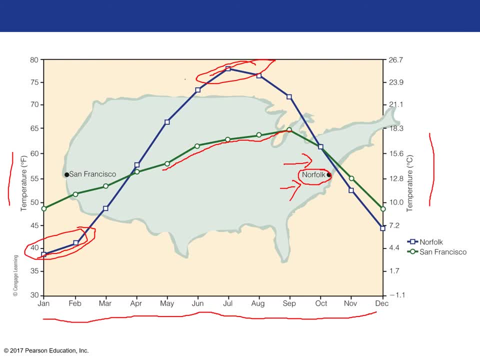 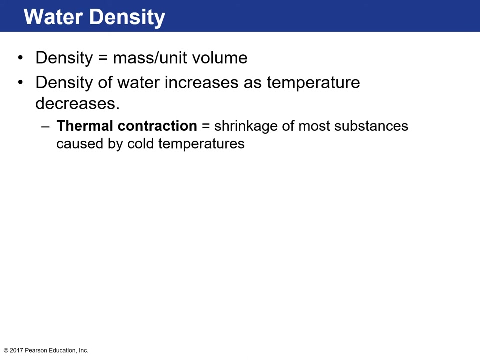 right, And in the summer it's really hot. So that range is really large, whereas the range from San Francisco is much smaller, So it helps moderate the temperature. So Norfolk Virginia has hotter summers and colder winters as compared to San Francisco. All right, another kind of 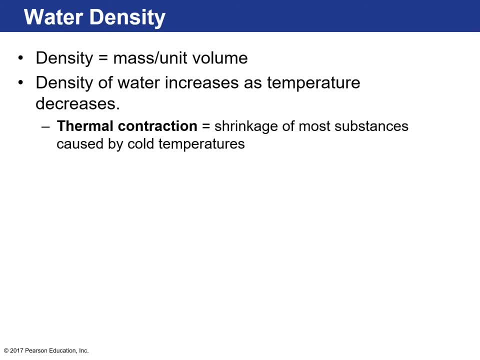 really unique property of water is its density and how it changes when it goes through phase changes. Density is mass per unit volume, And so the density of water increases as temperature decreases. So if you start like cooling water down, its density will increase And that's called thermal. 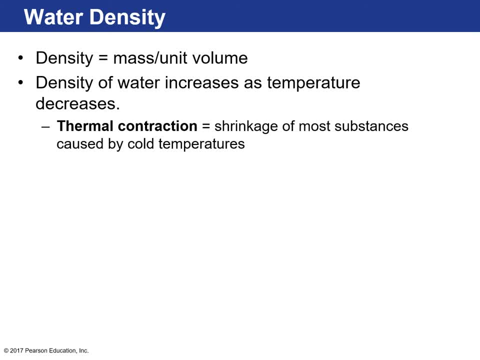 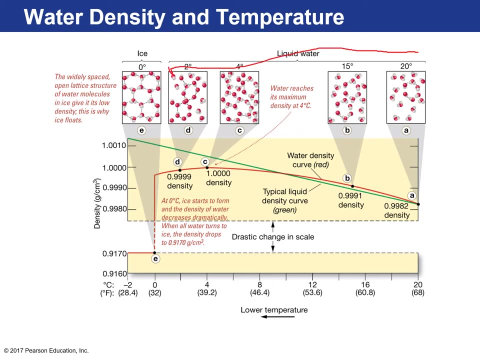 contraction Happens with most substances. We call it shrinkage. It kind of tightens the molecules together when you cool it down, Okay. But something unusual happens with water. Okay, So when you're going from liquid water to ice, okay, forming that crystalline substance, something very unique happens. So if you look at this, 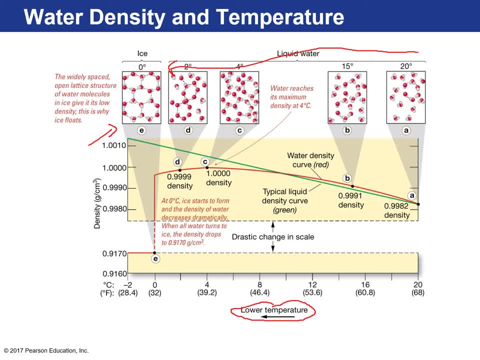 down here at the x-axis. that's temperature. So if we're going in this direction, we're decreasing the temperature, right And predictably. the red curve here is water. So as you decrease temperature- this is the y-axis- is density. So as you increase, decrease. 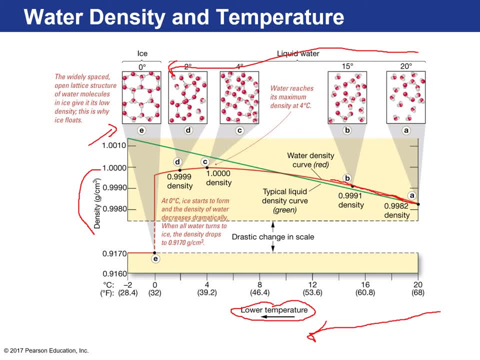 this is temperature. Density increases, it starts increasing, But then all of a sudden it kind of plateaus, Do you see that? And the colder and colder it gets density kind of plateaus to these areas c and d And then there's a big decrease or a jump in density as you go from liquid water to ice And so down here, this here E would be ice. That's the density, That's, if you're gonna go across once, you're gonna get into inner quisatula and there's something that happens, But uhTrust. I just I don't know if I've got it myself, but if we're gonna go through um any foi, a temperature it can happen, and also when. if I expect some kind of loss, then suddenly it gets cold, But make sure. 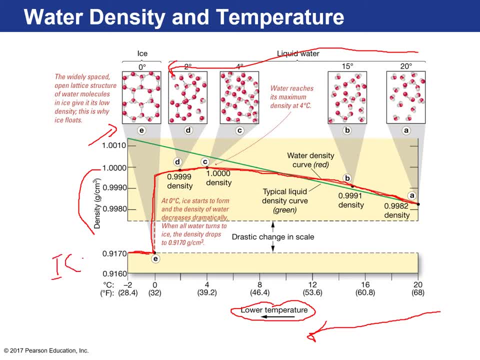 bear in mind that this excitedness doesn't happen in your head, Because if you think of so many things, that that's the density of ice, right? so the density of ice is less than that of water, and that's why ice floats. it seems totally normal, right like because you 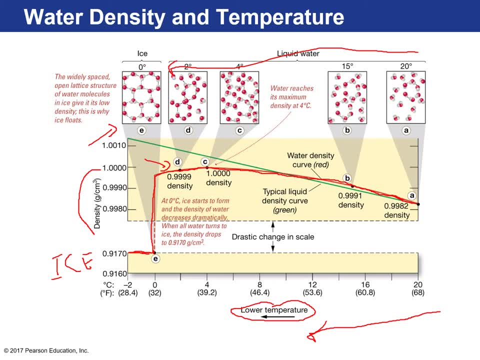 drink ice water. all the time you get a glass of water, you put ice in it, the ice floats to the top. that is weird. that is very strange. in terms of substances on earth typically, this green line is what normal substances. as you continue to decrease temperature, density will continually increase, even when it turns. 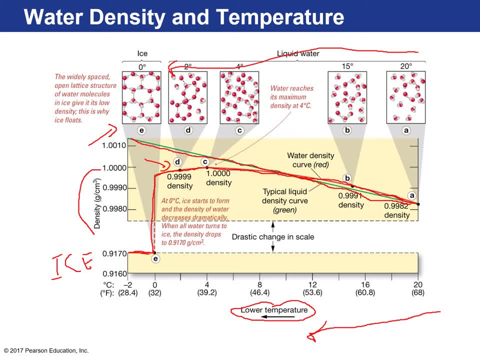 into a solid like say you have. let's just say you have liquid iron. let's say, and you have liquid iron, but then you have it's cooling down and then there's solid iron. within that liquid iron, the solid iron will sink amongst all the other liquid iron and sink to the bottom of. 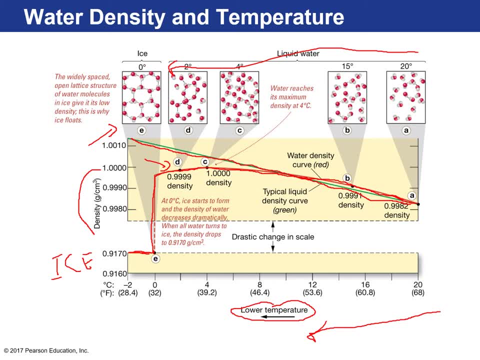 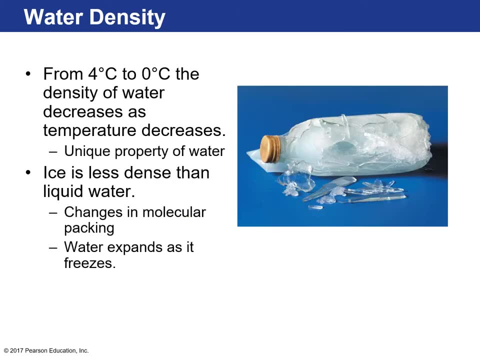 or whatever you know, heating it up in, okay. so that's, that's strange. ice floats- very strange, okay. another unusual property of water is that it actually expands by about nine percent when it freezes. so what happens is the way it forms that crystalline three-dimensional structure. it actually, it forces the 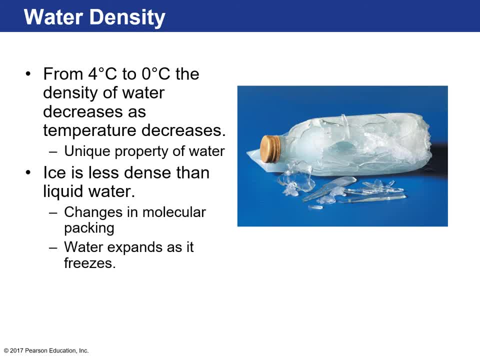 molecules to expand outwards, okay, and so it changes the molecular patent packing and then it expands water as it freezes. so I'm sure this has happened to you. maybe you had, maybe you were like, oh, I want a cold water, and you put it in the freezer but then you forget about it. 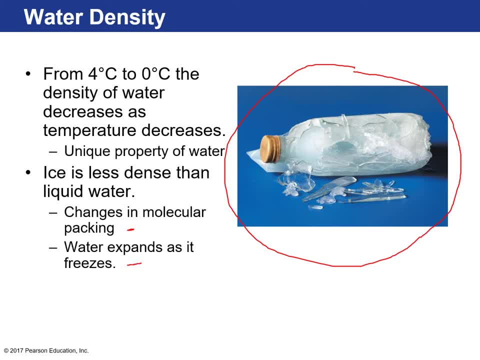 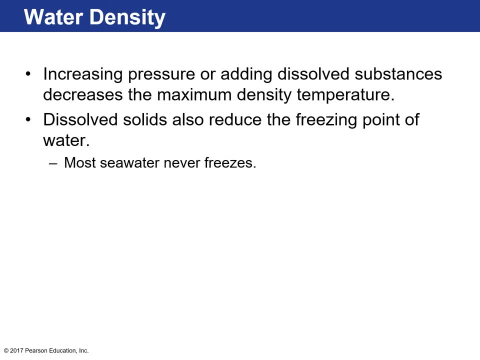 and then you go back in the water expanded and it busted the the bottle that it's in. okay if you increase pressure on water or adding dissolved substances, meaning like things like solids, like salt. if you add salt to it, that decreases the maximum or it increases its density. if 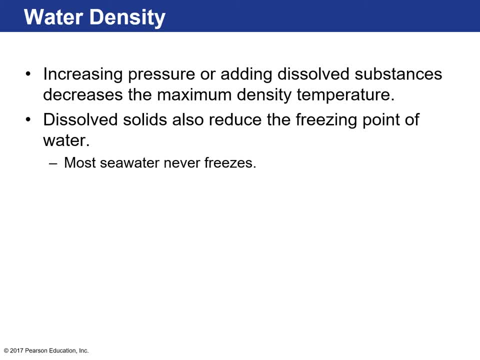 you add more dissolved solids in it. okay, dissolved solids also can reduce the freezing point of water. right, and that's why in cold places, people salt the sidewalks, because that lowers the freezing temperature of water itself and you won't get water or ice forming on sidewalks, or 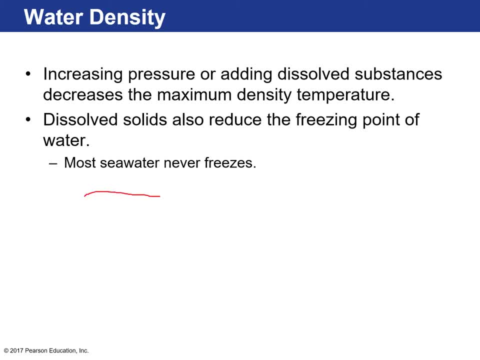 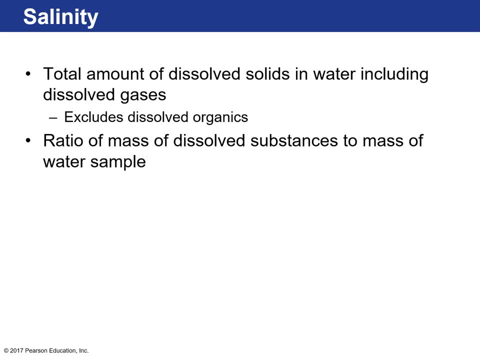 on roads And so on Earth. most seawater never really freezes because of the dissolved solids that are found in it And those dissolved solids that are in ocean water we refer to as salinity. That's the total amount of dissolved solids. okay, The ratio of the mass of dissolved substances. 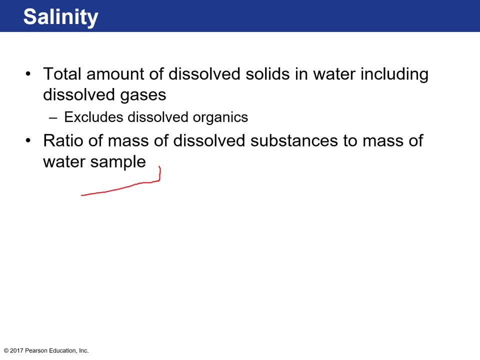 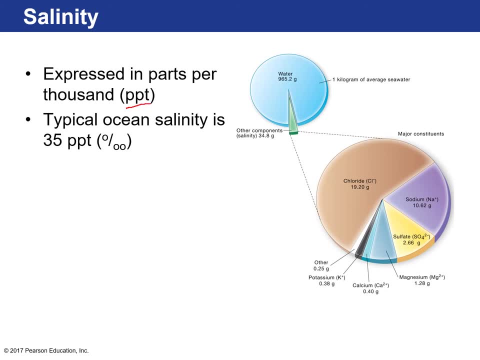 to the mass of a water sample is the salinity, And we typically express it in terms of parts per thousand or PPT. So the average ocean salinity is about 35 parts per thousand And it's easy to remember because parts per thousand if you have a kilogram of seawater, which is a thousand. 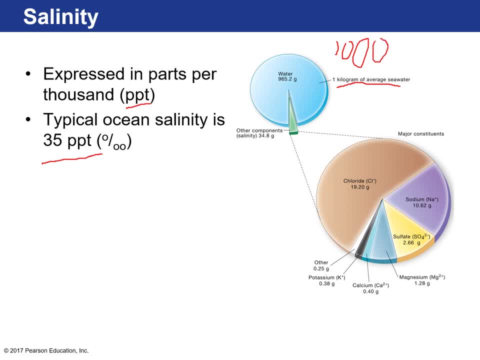 grams, okay, Whoa, okay. A thousand grams of seawater, that means 35 parts per thousand will be dissolved solids. So that means that there's approximately 35 grams of dissolved solids in seawater. okay, So if you had a kilogram of seawater, let it evaporate away. 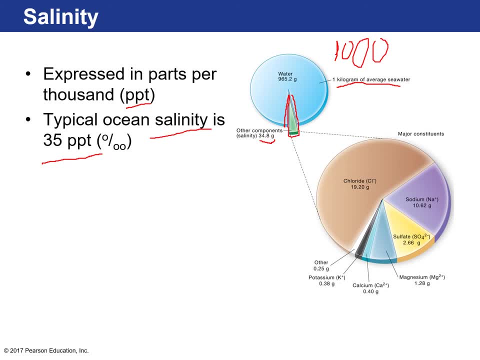 you'll have left behind approximately 35 grams of substance. okay, If we break that down into what those components are, here are the ions: Chloride makes the majority, and then there's sodium. Those typically bond together, make sodium chloride. That's salt. 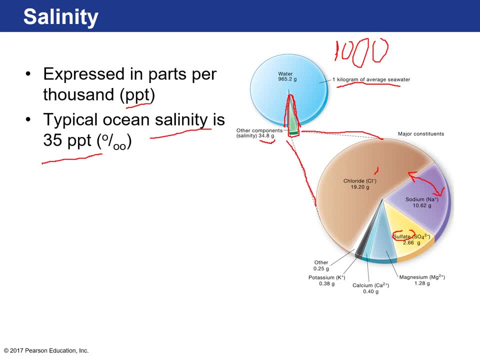 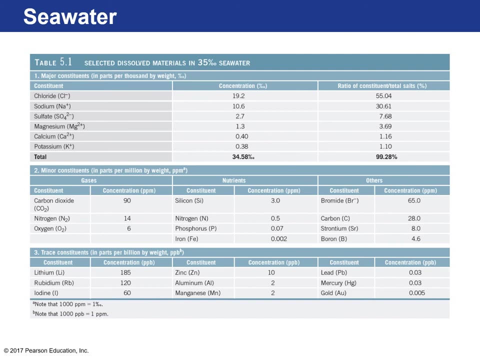 so it's mostly salt, But then there's sulfate, there's magnesium, a big portion calcium, potassium and then a slew of other elements that make up the rest. Here's an example comparing the salinity in seawater. Here are the different constituents. okay, Some of the minor constituents. 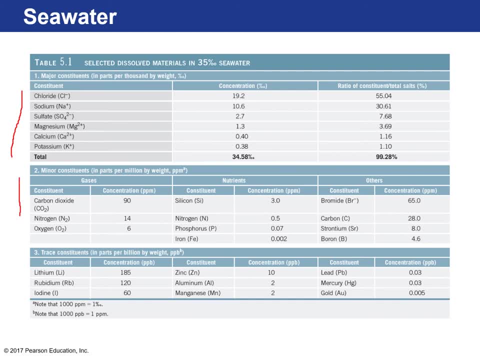 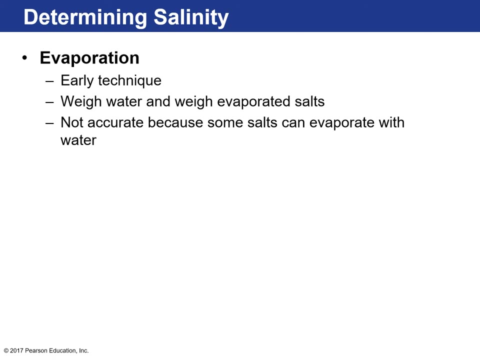 in seawater: Oxygen, nitrogen, carbon dioxide, dissolved gases, nutrients, and then the trace constituents- okay, Stuff, that's in really small amounts, okay. So how do we determine salinity? One way is evaporation, As I mentioned before. that's a very early technique. You just get some seawater. 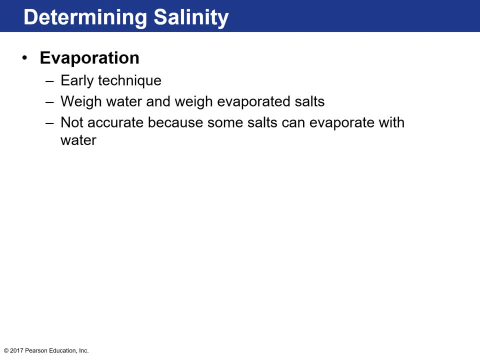 let it evaporate away and then you know, find out and, like you, can measure the weight of the water. then it evaporates away and then measure what's in the water. So that's a very early technique. That's what's left behind. That's a way of doing it, But it's not too accurate because some salts 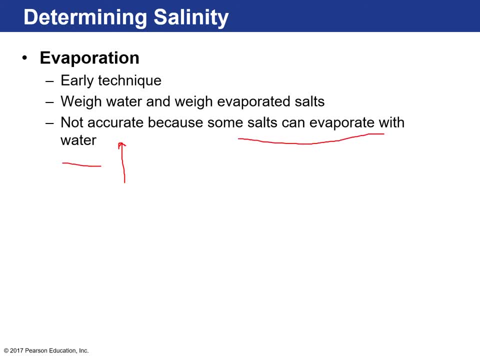 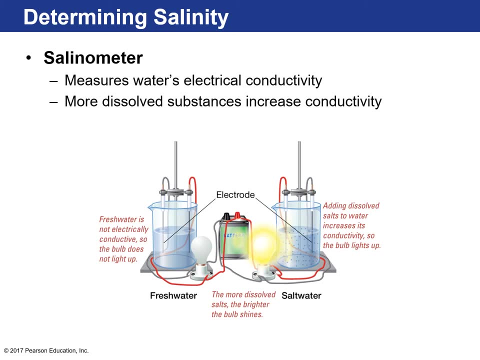 evaporate with the water. So then you're actually underestimating the salinity of the water itself. So later on other things were developed, like a salinometer. This measures the water's electrical conductivity, So the more dissolved substances you have in the water, the faster or 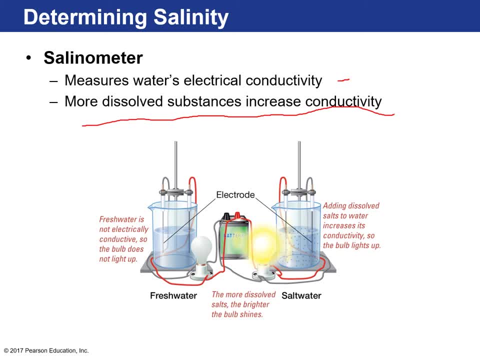 more efficient the water is, So that's a way of doing it. So, for instance, like: for example, let's say you have some seawater and then you put a battery in it and you put electrodes in water, and you put electrodes in the water and you put electrodes in the water. 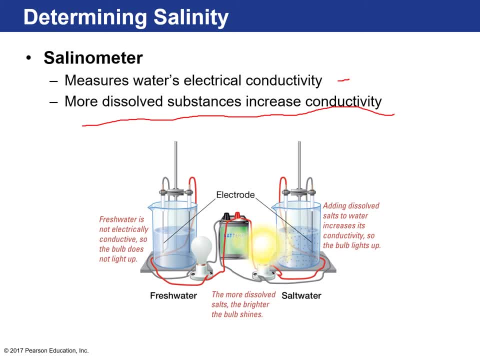 okay. So for example, say, you attach a battery and you put electrodes in water. if fresh water is not electrically conductive, so this bulb wouldn't light up, but if you have seawater there are a lot of dissolved solids in it. that helps transmit those electrons through it and makes it more. or 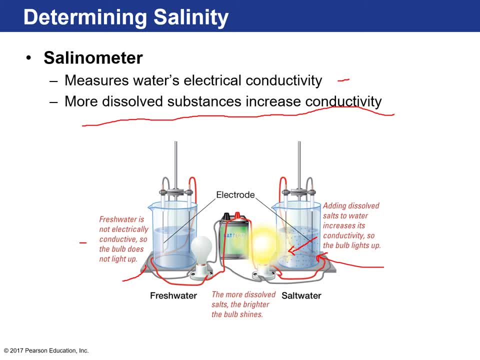 increases the conductivity. So the saltier the water itself, the more conductive it is. So that's a way of doing it. That's a way of doing it, Alright, so I'm going to go back to the next slide. So let's go back to the next slide here. 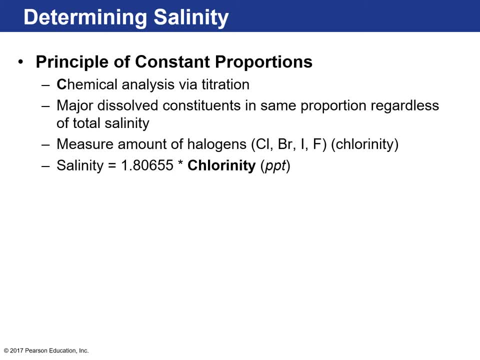 that's how a cylindrometer works. And then there's the principle of constant proportions, and this is analyzing the proportions of materials in ocean water via titration. I'm sure maybe you've seen that in a chemistry class. So the major dissolved constituents in ocean water remains in the same proportion. 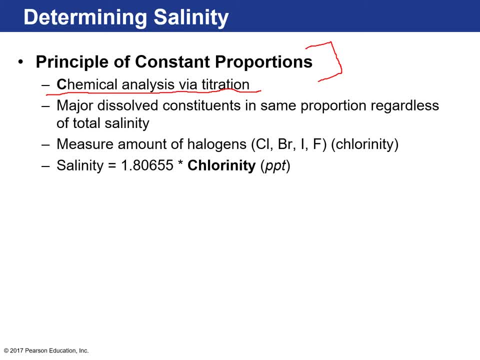 regardless of total salinity, Like, for example, I think sodium was about 25% of the dissolved substances in seawater. So you can go to a different area on earth where you find real or ocean on earth where you find really salty seawater. but 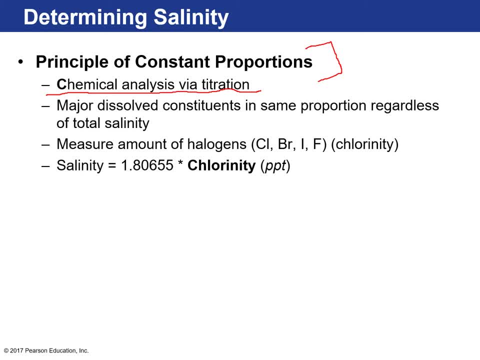 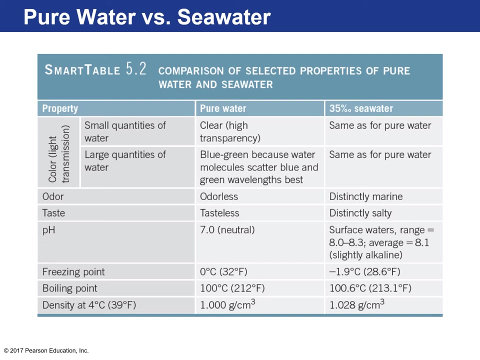 the proportion of that being sodium would still be 25%, versus other areas where you have input a lot of freshwater from rivers, The proportions of those dissolved solids remains the same. okay, So here is just an example of a comparison between pure water and seawater. okay, If you. 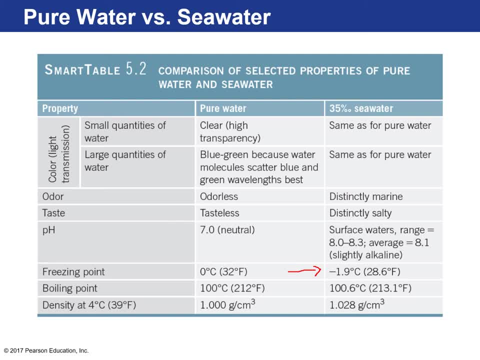 notice the freezing point is lower in seawater, so it has to get much colder as well, as the boiling point is just a little bit higher And, if you also notice, the density of seawater is larger than that of pure water, and that's because 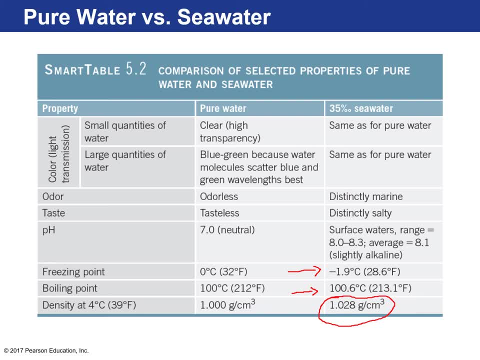 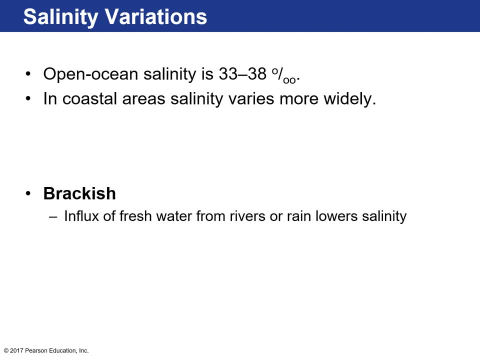 of all the dissolved solids that are in them. So in the inner open oceans the salinity varies between 33 and 38 parts per thousand. That's in the open ocean, In coastal areas, meaning like closer to the continental shelves all. 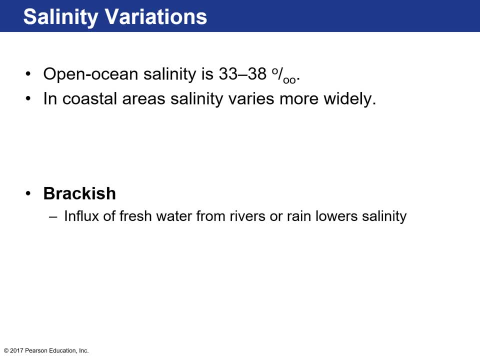 right shallower water, coastal areas. the salinity can vary more widely, meaning that if you've enclosed areas where the evaporation rate is lower, then the evaporation rates are high. you'll have higher salinity. Or if you have a lot of. 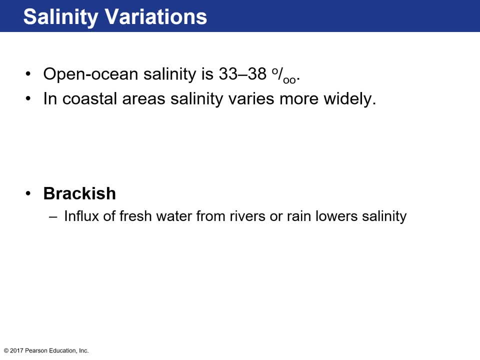 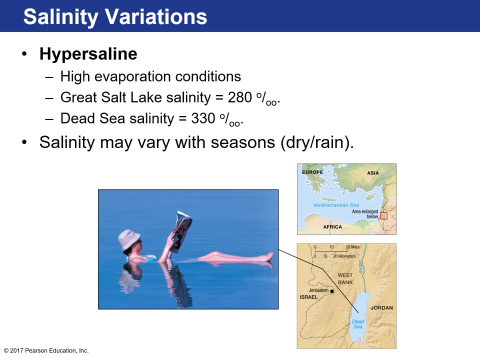 rivers, dumping out fresh water into the coastal areas. that will lower salinity And those mixes of fresh and salt water we call brackish water. okay, That typically lowers salinity. There are special areas that have really high salinity. We refer to them as hypersaline And what that means is usually it's like: 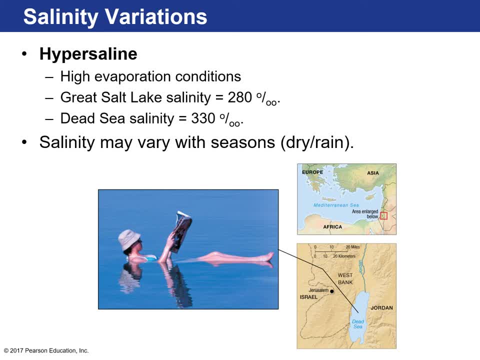 an enclosed area where evaporation rates are really low, And that means that the evaporation rates are really high, like the Great Salt Lake has, the water there has a salinity of 280 parts per thousand, And the Dead Sea, which is found here, 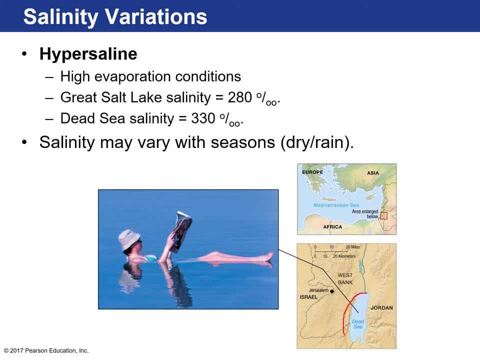 between Jordan and Israel. this area here very dry, really high evaporation rates. the salinity there is 330 parts per thousand, So it's almost that's about ten times saltier than the regular ocean, And so what that means is: 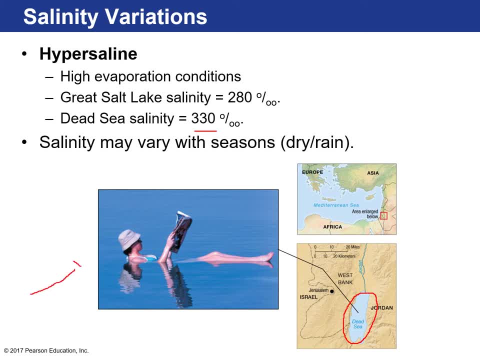 if you ever go here. it's so salty. the ocean water is so dense that our density doesn't really change that much, so you can float in the Dead Sea without even swimming, And that's because the water is so dense relative to you. you become like 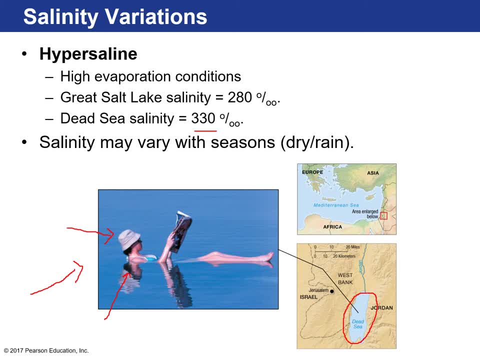 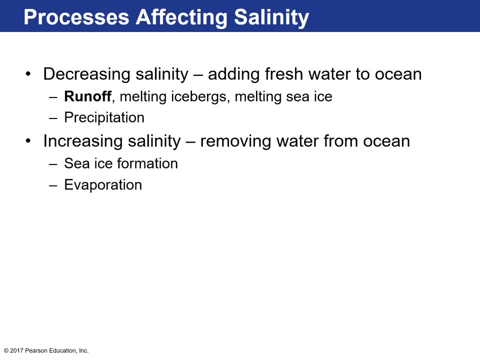 a boogie board and you can just you just float to the top very easily because the water is so salty. So this woman is really coolly reading a newspaper without worrying sinking in the water because the water is so dense. Okay, so what are the? 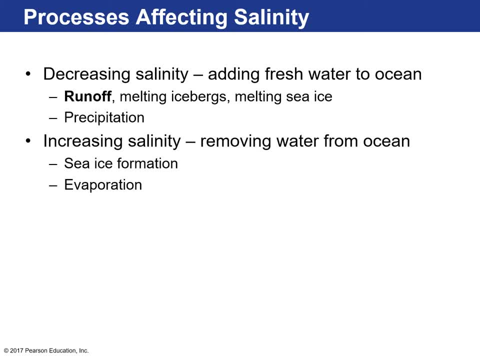 processes that affect salinity. When you have decreasing salinity, typically that means adding fresh water to the ocean- rain or precipitation will lower sea surface salinity runoff from rivers. if you have icebergs that are melting or sea ice melting into the ocean, that will all lower salinity. The things that 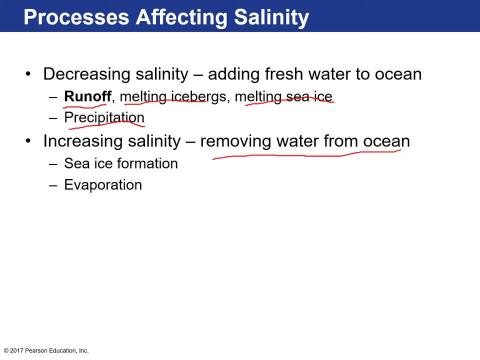 increase salinity. essentially, what that means is: if you're removing water from the ocean, remember, so you have the ocean. evaporation is basically taking water molecules and moving them into the gas phase, transferring heat. that will increase salinity. Alright, so that evaporation is an example of that In cold. 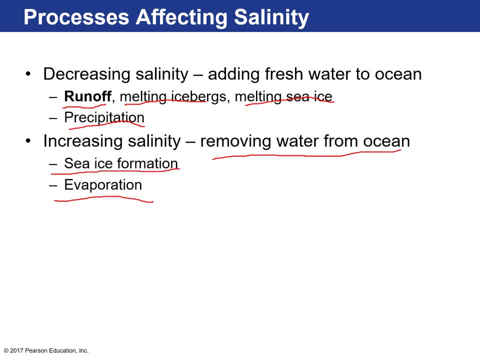 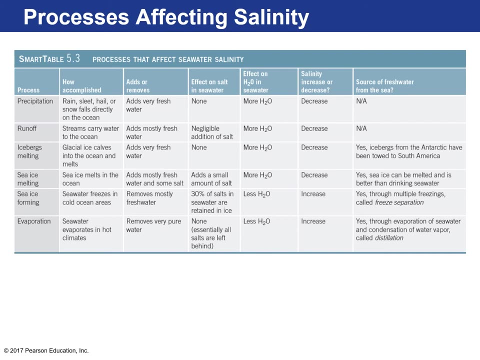 areas where sea ice forms at the surface, ice itself does not include any of the dissolved solids in it in its structure. so when ice forms, it's like removing water from the ocean, so the remaining water that's left behind, because it's saltier as a result. So here are those processes here and this is 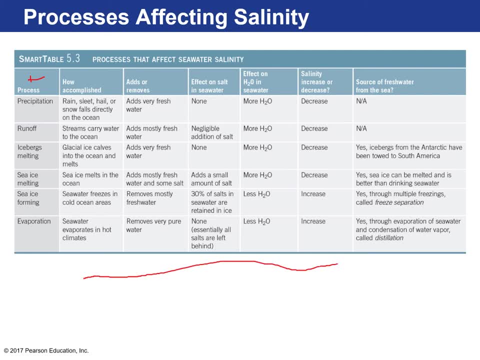 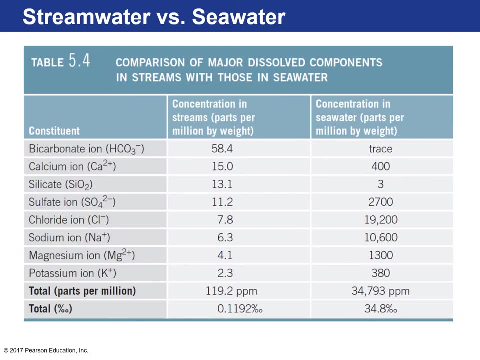 how they affect sea water salinity. you can review this later in more detail. Alright, here are. this is a comparison of river water to sea water. Okay, here are the different constituents in the water. or dissolved solids. okay, Pure water would be closer to having not too many dissolved solids, but 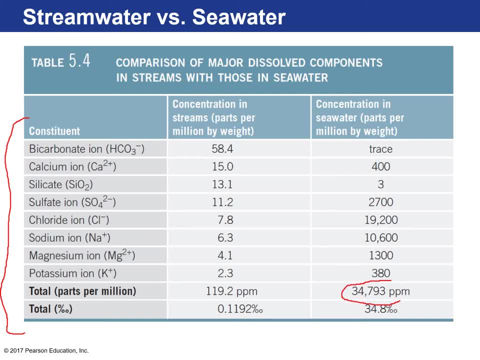 look at sea water has 34,000 parts per million, or around, on average, 34 parts per trillion, of dissolved solids in them, and it's mostly chloride and sodium. That's why it tastes nasty. when you taste sea water, I know accidentally, maybe a wave. 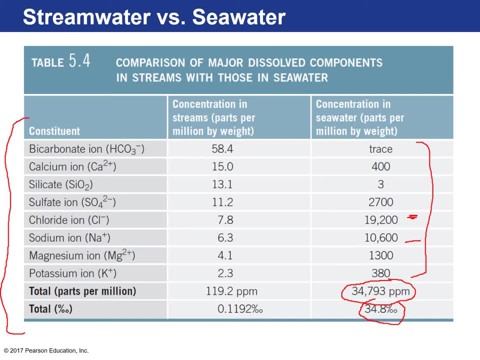 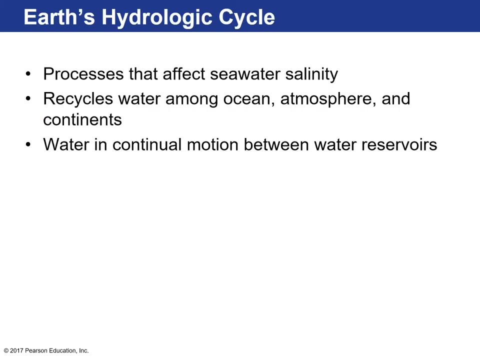 hit you in the mouth and you just gagged, tasting sea water- Yeah, river water. on the other hand, much less dissolved solids in it, not even one part per thousand. it's only 0.1 parts per thousand. Okay, so let's understand how water moves through all. 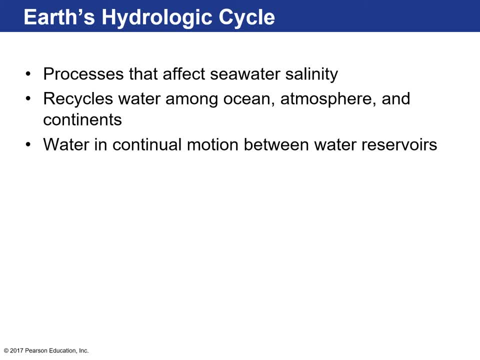 the different environments on earth. we call that the hydrological cycle. This also affects sea water salinity. it helps recycle water from the ocean to atmosphere, to continents, to groundwater, and water is in continual motion because it can move through all three phases and be transported with atmospheric. 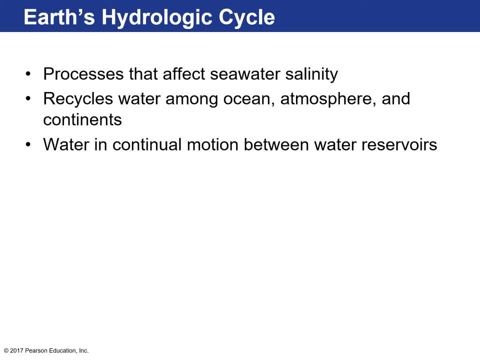 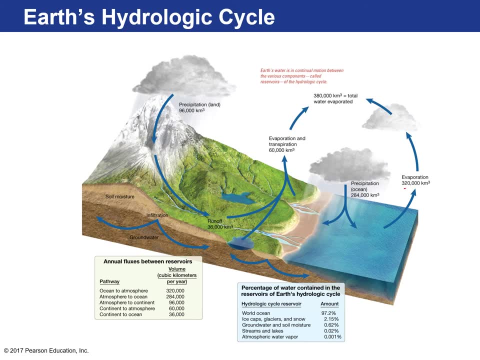 winds, it can get everywhere, and essentially, water just hopping from different reservoirs. Okay, so in the ocean, every year approximately 320,000 cubic kilometers evaporates into the atmosphere, and that evaporated water travels into the atmosphere, condenses and then falls down on rain as rain or 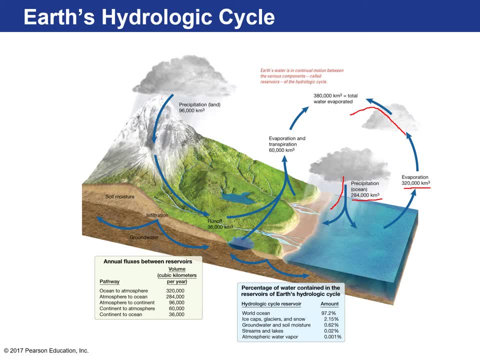 precipitation as snow. Most of that- 284 cubic kilometers- just falls right back into the ocean. okay, About 96,000 cubic kilometers will precipitate on land as rain or snowfall, and then that water will run off and return into the ocean or evaporate back. 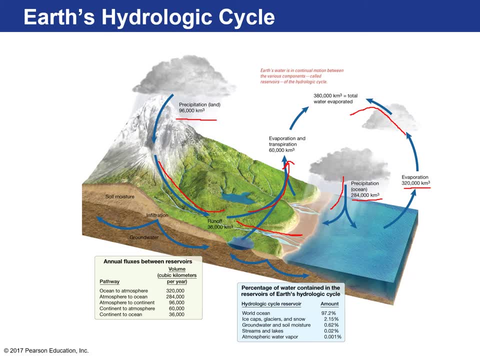 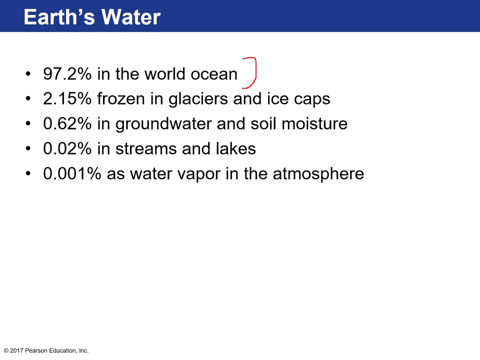 into the atmosphere. So that's oh. and some of that water infiltrates down into the groundwater. so that's the fate of water as it kind of travels through our entire environments, Our water. most of it is found in the ocean, about 97.2%. The rest is found in. 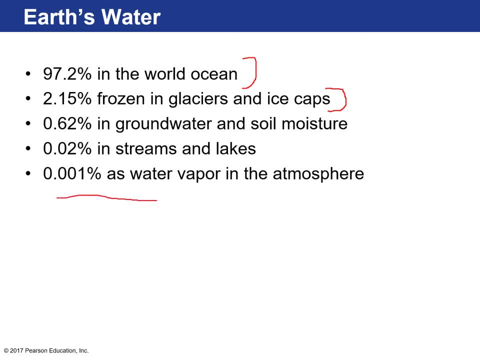 glaciers and ice caps, and then all the water that's in the atmosphere, streams and lakes, Lake Toho, Lake Titicaca, all the groundwater that's less than 1%, less than 1% of global water. okay, So most of the water is found in the 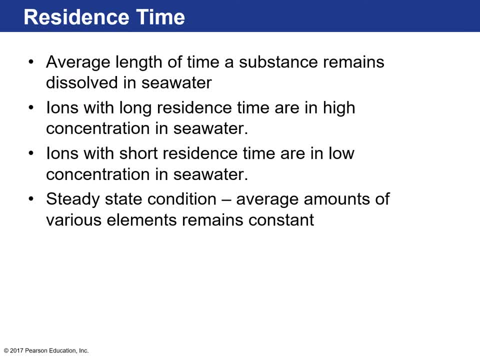 oceans and in glaciers. Residence time is the average length of time for a substance to kind of remain dissolved in seawater. Ions that have high residence time in the ocean typically are higher in concentration Dissolved ions that are in the ocean with short residence times typically. 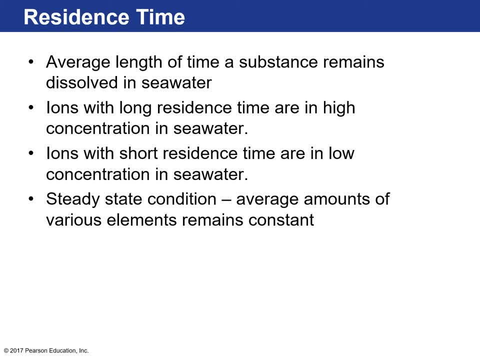 mean that they're in lower concentration, And what that means is that they get pulled out for some process. some process pulls them out of the ocean itself, But the ocean's in the steady state condition and that's the average amount of various elements kind of remains constant. 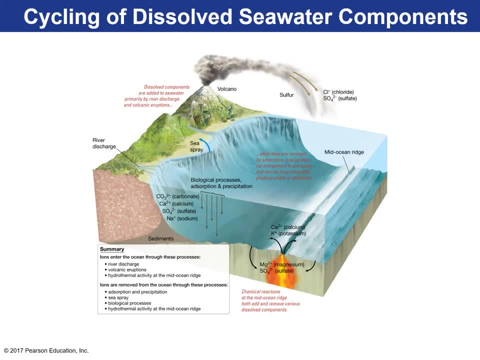 in our oceans And this is how different materials cycle through our oceans. okay, Here ions that enter the ocean. through these processes, we have rivers discharging. rivers go into the ocean and discharge a lot of dissolved solids- okay, into the ocean. And then we 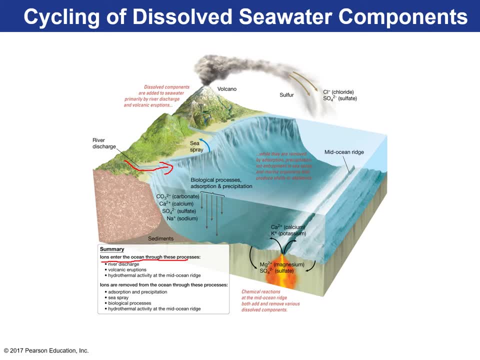 have a lot of water that goes into the ocean and that's typically weathered material, rocks from land, Volcanoes can erupt, and this material delivers sulfate and chloride into the ocean. okay, And then, finally, hydrothermal activity provides a lot of calcium and potassium. 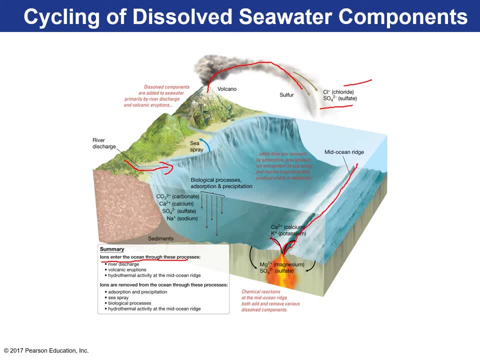 So these are volcanic areas at the bottom of the ocean, mid-ocean ridges. There's a lot of circulating ocean water here and a lot of ions are delivered to the ocean through these three processes, And then ions are removed from the ocean by absorption or precipitation. 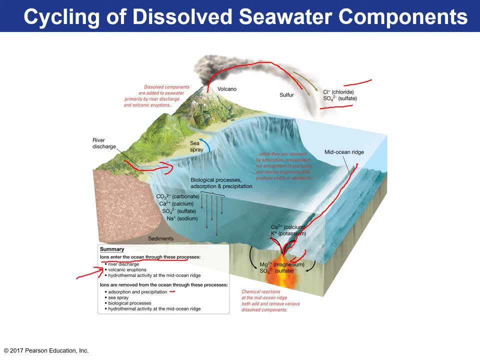 so things directly precipitating out of the water. Here's some absorption. some magnesium and sulfate are kind of almost like deposited and interacting with the rock in these hot volcanic areas. Sea spray biological activities, so carbonate, calcium, sulfate and sodium. 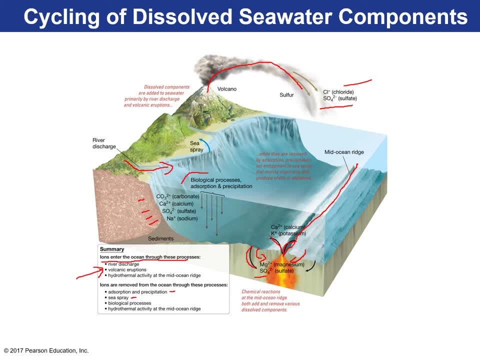 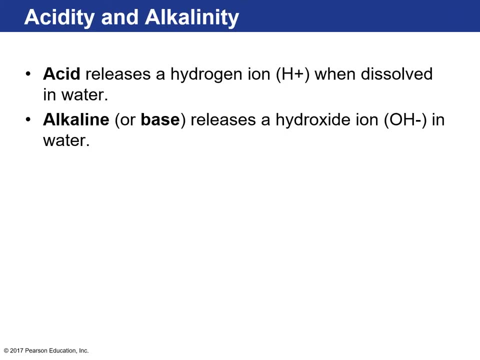 are part of this process, And then also the hydrothermal activity at the bottom, The ocean's acidity and alkalinity, or that balance we refer to as pH, is very important, And acid is a solution that releases a hydrogen ion, H+, when it's dissolved in water. and 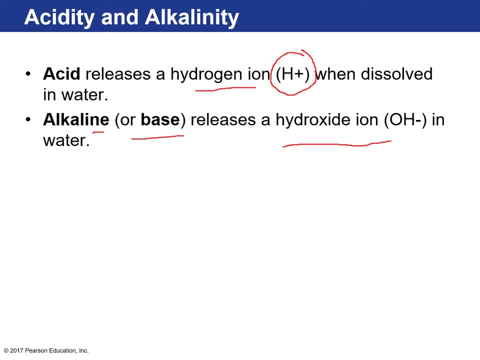 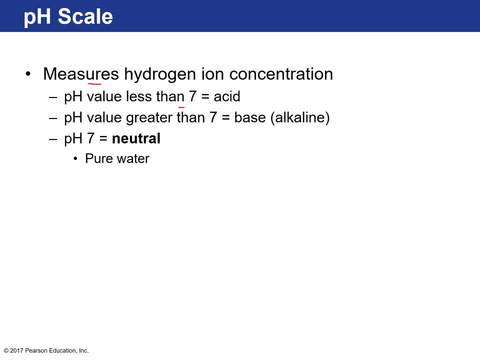 an alkaline or base. that's a solution. that's in a solution that releases an alkaline, well, releases the hydroxide ion in water. Okay, and then pH scale is what we use to measure that. Any pH value that's less than 7 is considered an acid, so lower. 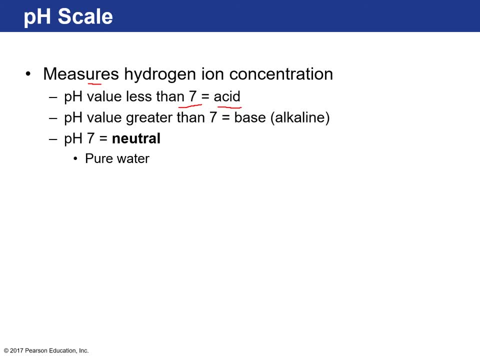 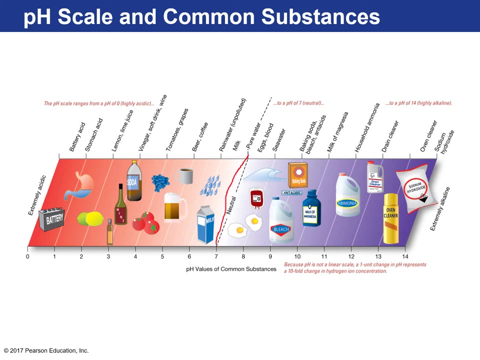 numbers are acid or more acidic, and pH values that greater than 7 are basic or alkaline. Pure water is neutral at 7.. So here are some common substances on that scale. Here's pure water, that's neutral, Milk, rainwater. 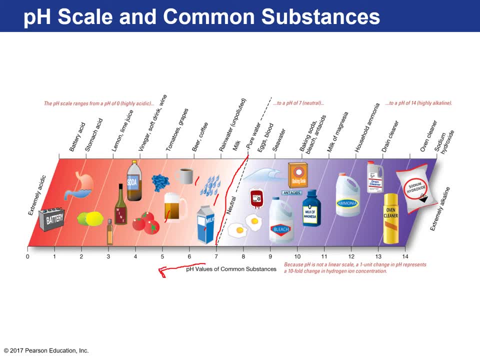 coffee, beer. that's more on lower on the scale, so it's more acidic. Tomatoes and grapes are kind of acidic and then you go down to the worst: is battery acid over here. that's really acidic. If you go in the other direction, more alkaline. 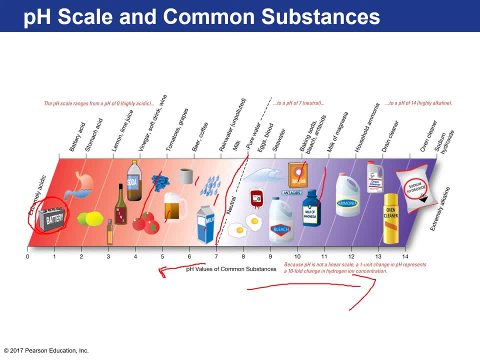 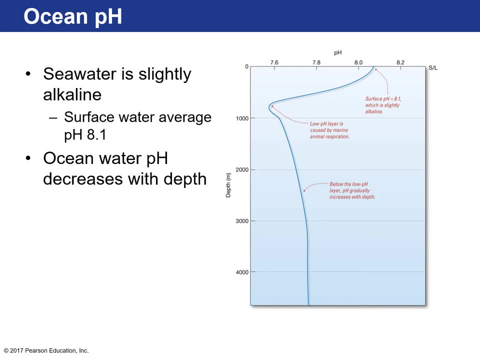 materials: baking soda, milk of magnesia, household ammonia, drain cleaners. those are more basic, So the pH in the ocean varies from the surface as compared to deeper ocean water. So if we look at this scale here, 0 to about 4,000 meters, this is ocean. 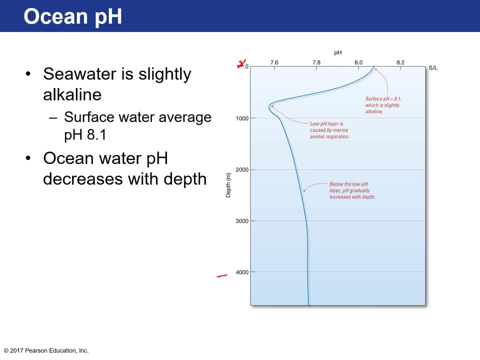 depth. So this is the surface, and then this is approximately 4 kilometers beneath the surface, And then up here is the pH scale. So surface ocean water has a pH of about 8.1.. Okay, so it's. it's more alkaline than pure water, But as you go to deeper and deeper levels, 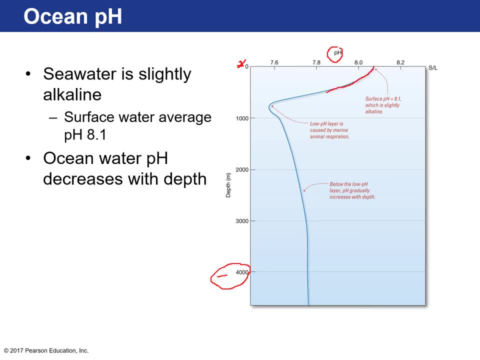 within the ocean, the it becomes more and more acidic. okay, And the reason is this really low pH layer here, right before you hit one kilometer of depth- is caused by marine and animal respiration, And then, as you gradually get deeper and deeper, this becomes just a slightly. 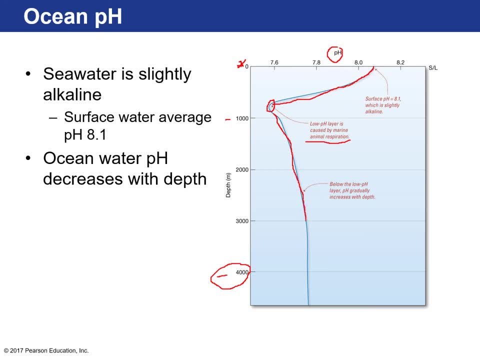 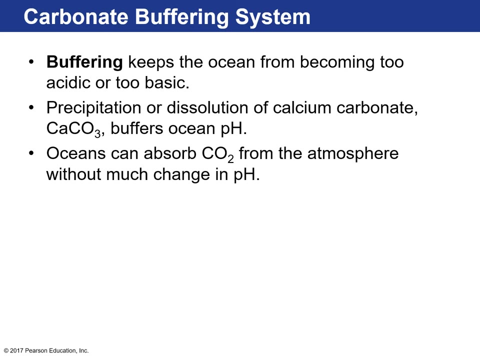 bit more basic as you go deeper and deeper, But still deeper waters tend to be more acidic than surface waters. Then there's the carbonate buffering system, And buffering essentially keeps the ocean from having wild swings in alkalinity or acidity, And what that essentially means. 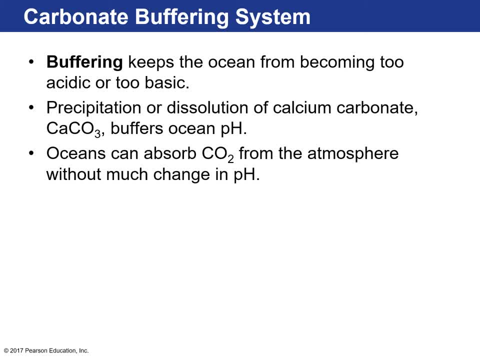 it kind of keeps it balanced and keeps the chemical reactions from going too far in one direction. Okay, So what happens is the precipitation or dilution of calcium carbonate, which is this here- really keeps in check or stabilizes ocean pH? So what happens is it's. 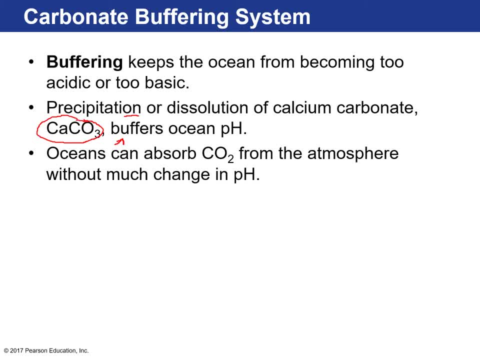 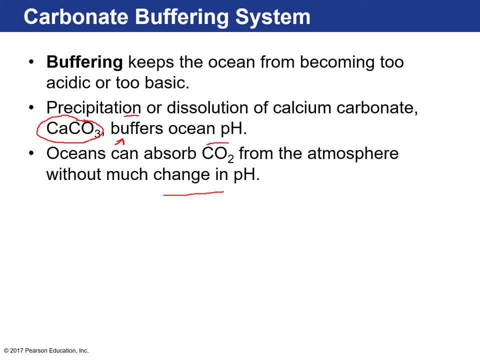 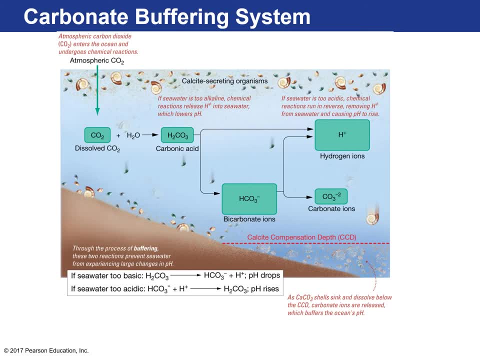 of CO2 from the atmosphere, there won't be big changes in the pH. Let me show you the diagram. This might make more sense. Okay, So as atmospheric carbon dioxide enters and is absorbed by the ocean and it becomes dissolved CO2, you add that to water and you make carbonic acid. So if seawater 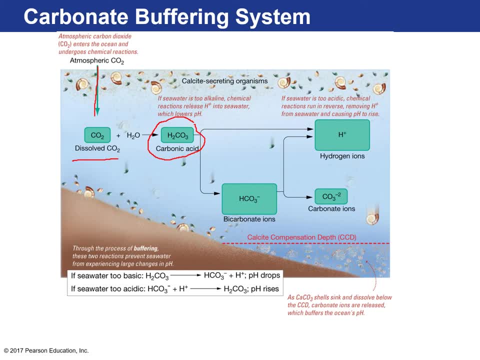 too alkaline, the chemical reactions start to release the hydrogen into the seawater, and that will lower the pH. now, on the other hand, if seawater becomes too acidic, the chemical reactions will run in the opposite direction. okay, so then here: the bicarbonate ions will combine with the hydrogen free ion, and then 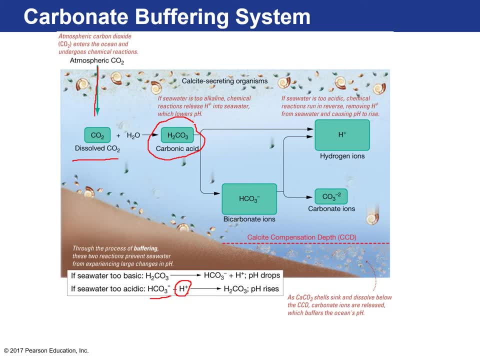 create carbonic acid and pH then rises. so these two equations are our chemical reactions are occurring simultaneously and it kind of balances the- the oceans- acidity okay, and the the- the calcium carbonate that's in the ocean in large part is created by calcium secretion organisms. so these are the. this is the material that precipitates and dissolves. 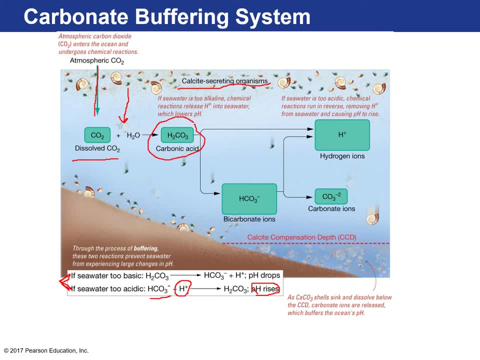 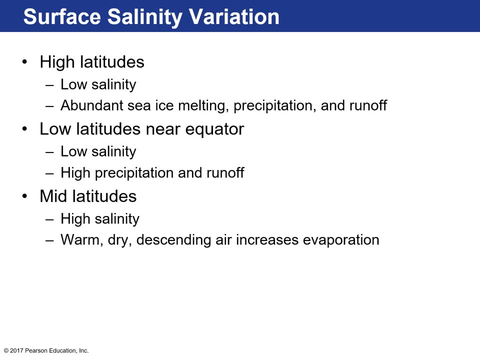 and kind of runs these reactions and buffers the whole system. so surface salinity- surface meaning if you're on the surface of the ocean, that varies- or open ocean surface salinity varies depending on where you're located. if you're at high latitudes, you typically have low salinity and the reason is 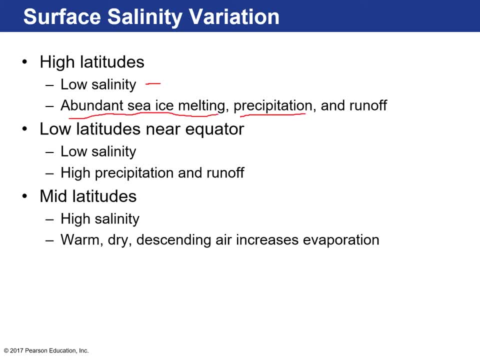 because there's abundant CIOs melting, precipitation and runoff going into the oceans. at lower latitudes you also have lower salinity and that's because there's a lot of rain and a lot of runoff and mid latitudes. these are the high salinity latitudes and that's. 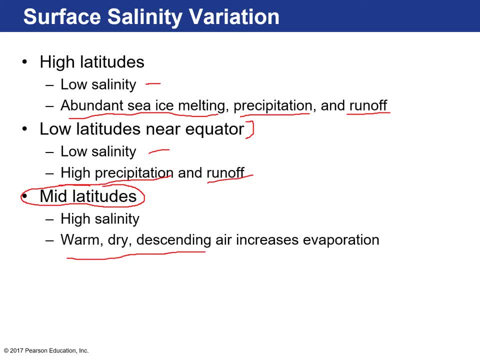 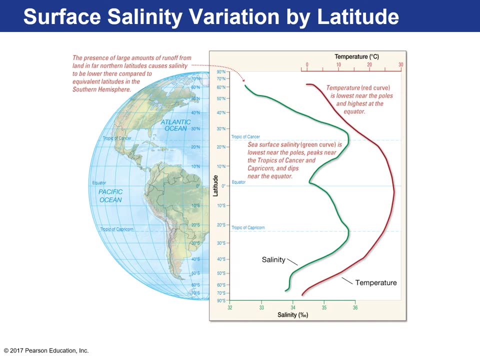 because there's a lot of warm and dry descending air coming from really high altitudes in the atmosphere and that increases evaporation, which leaves the remaining ocean water very salty. okay, so if we look at a globe and we check out the here's, the temp, here's- 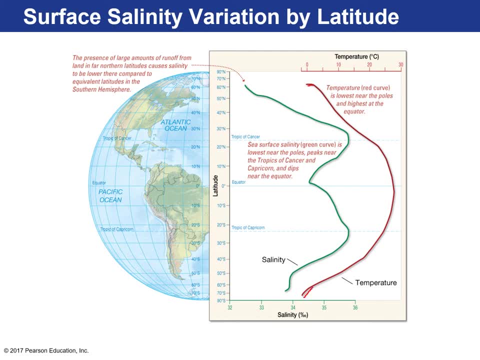 temperature right. so from pole to pole it's it's very cold and then as you approach the equator, becomes very warm on average. so you go from low salinity, high latitudes, to low salinity, to high latitudes, to the equator. you typically have low salinity, and then these are the at the Tropic of Cancer and at the 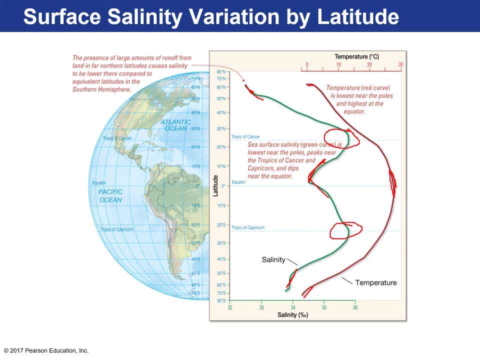 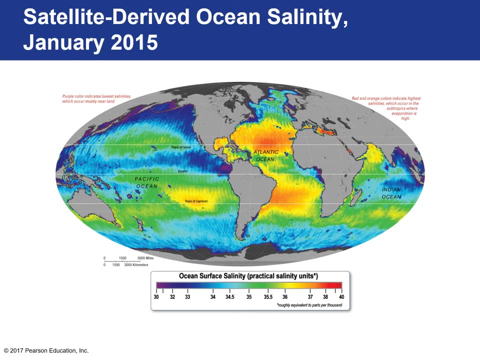 Tropic of Capricorn you have high salinity and that's because evaporation rates are really high. so here's a satellite derived ocean salinity map of the globe and it confirms what we just saw is that at the Tropic of Cancer, these latitudes and Capricorn, we have higher salinity than 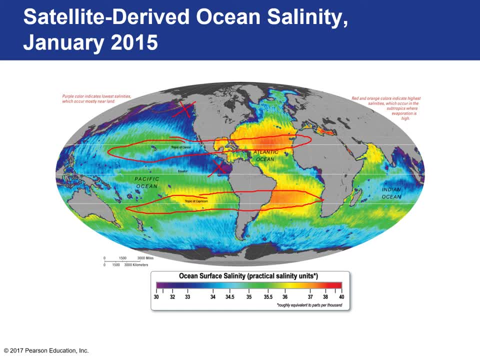 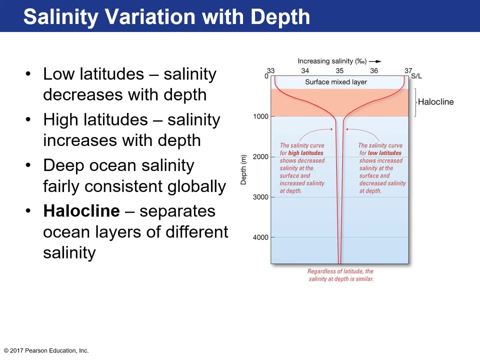 than here at the equator and at the closer to the poles right. this is ocean surface salinity. so, whatever you see, an orange and red has higher salinity. lower salinity would be in these kind of purples and blues. So how does ocean? 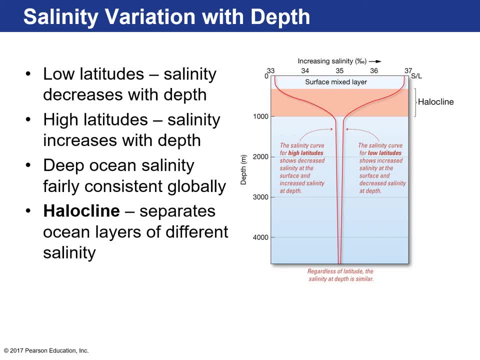 salinity vary with depth. Here it doesn't really break down mid latitudes- We're going to do that in another lecture- but at low latitudes typically salinity decreases with depth. Okay, so here is the low latitude the salinity curve for. 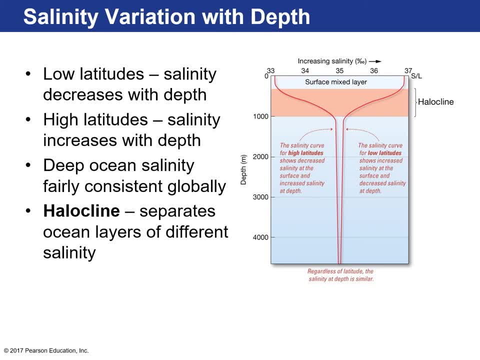 low latitudes. So that shows increased salinity at the surface and it decreases with depth. So this is the surface, here is salinity on the x-axis, here's depth. so you're going down deeper. What happens is you're going down deeper. what happens is: 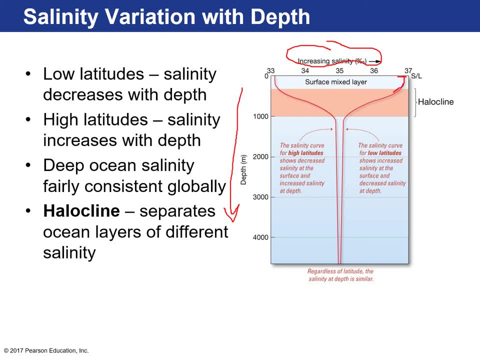 you're going down deeper. what happens is salinity is kind of constant, and then you see here a drastic decrease in salinity. At high latitudes you start off with low salinity. I'm sorry, this should say mid latitudes, mid latitudes. At high latitudes you start off with low. 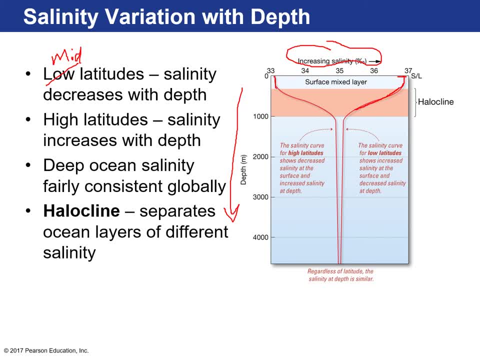 salinity and then as you get to right around like 300 meters, then salinity increases drastically and then once you go beyond 1 kilometer, at both mid and high latitudes, the salinity kind of levels off and kind of they almost close in together the deeper and deeper you go, And so what this creates is right here. 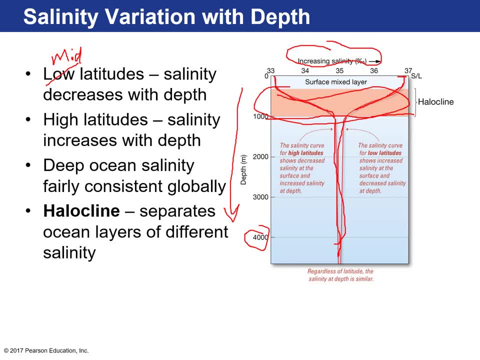 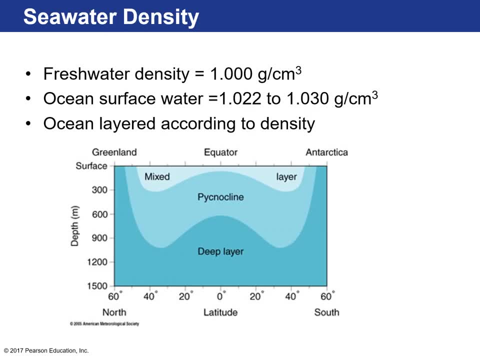 there's this layer called the halo climb and that separates different ocean layers based on salinity and density. So fresh water or pure water has a density of 1 gram per cubic centimeter. So fresh water has a density of 1 gram per cubic centimeter. 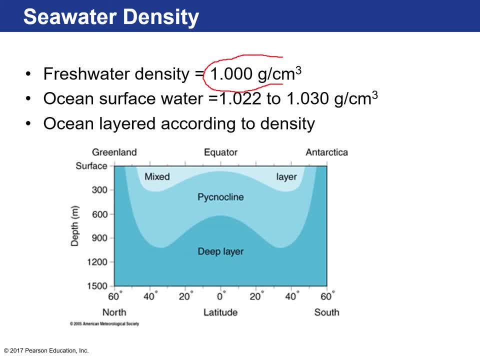 So fresh water or pure water has a density of 1 gram per cubic centimeter. Ocean surface water is denser and it because salinity varies and temperature varies, then the density varies as well. So that varies from 1.022 to 1.030 grams. 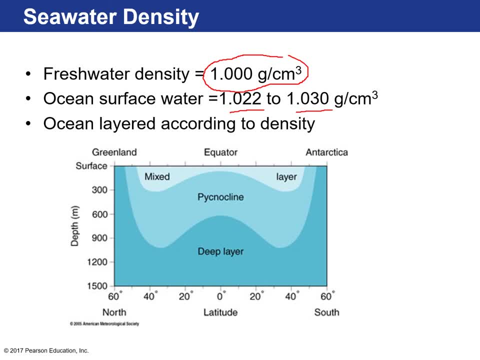 per cubic centimeter, And so what that means is that the ocean itself is layered, based on the density of water masses. So if we look at a cross-section of our ocean, okay, here's Antarctica right here and Greenland in the North Pole, and then 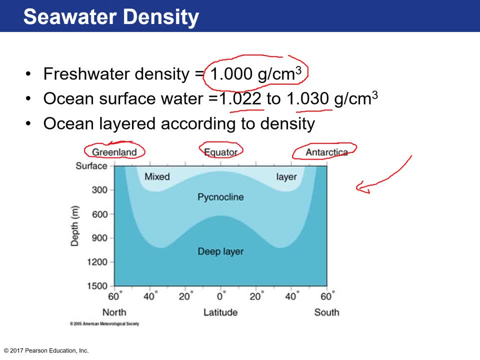 here's the equator. Okay, so we're looking at pole to pole cross section. here's depth. so surface down to really deep. What it creates is a three layered structure. We have this upper layer of very low density, warmer mixed layer. we have here, Then below that, 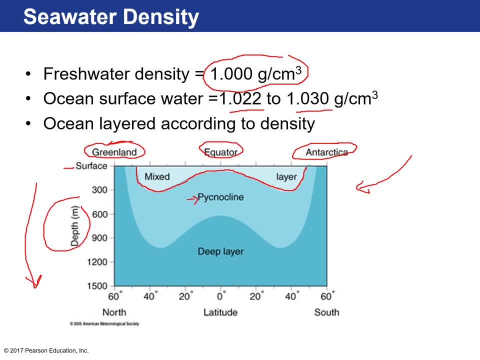 would be the halo climb or the pycnocline. we'll go into what the pycnocline is, But this is the second layer. Now, this is not the scale. the decline really isn't that thick. and then the last layer, which makes up the 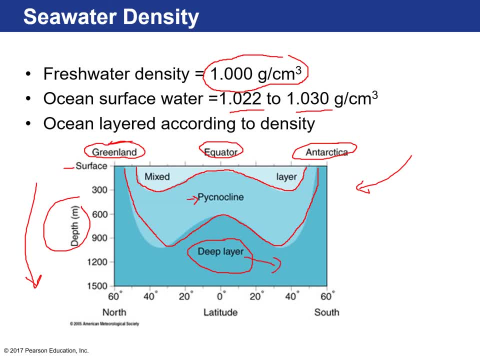 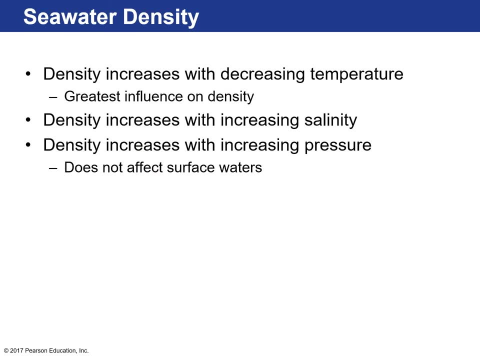 majority of ocean water is called the deep layer. okay, so density increases with decreasing temperature and that really has the greatest influence on density. okay so if you have member density equals mass over unit volume. okay so, if your temperature is going down, right, remember temperature causes shrinkage, so that would mean that the volume would decrease, right, which would 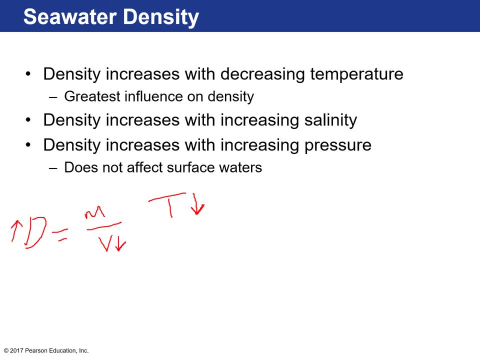 make this whole value go up. so density would increase if temperature decreases. now if, say, you had density over mass or volume, say you had instead temperature increases, temperature increase would mean that the volume is going to expand. so the volume expands, which makes this number or this fraction smaller, and therefore the density would decrease, alright. so 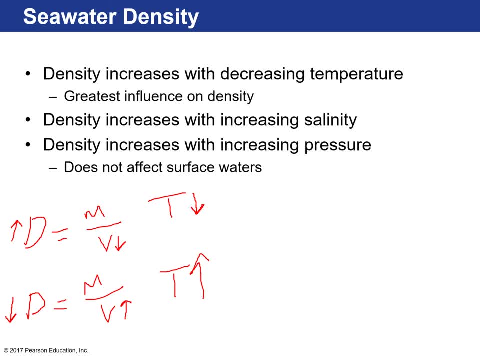 that's how temperature affects density: decreasing temperature, increased density, increase in temperature- that would actually decrease density. okay, if you have salinity, density increases with increasing salinity. okay, that's the example of the Dead Sea. if you have more salt in the water, that means it's denser and density also increases with pressure. what that means is the 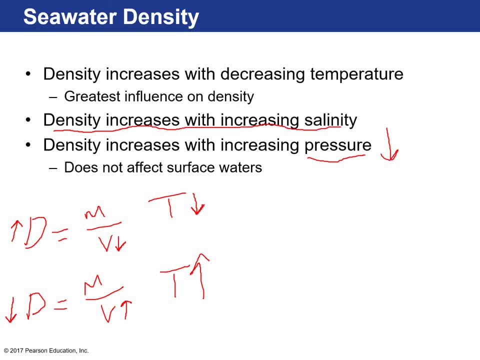 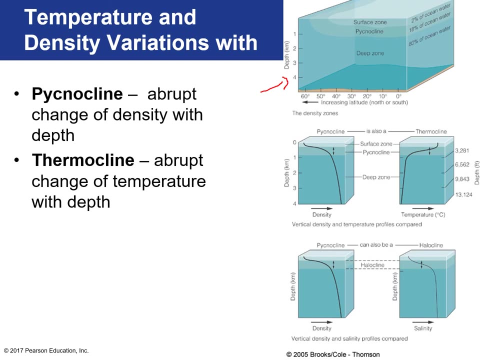 deeper and deeper you go beneath the surface of the of the ocean, the higher and higher pressure there is, and then the water becomes more dense as a result. okay, so let's take a look. here's a more accurate depiction of those ocean layers from density. there's a surface zone here, low density water at the surface makes up about. 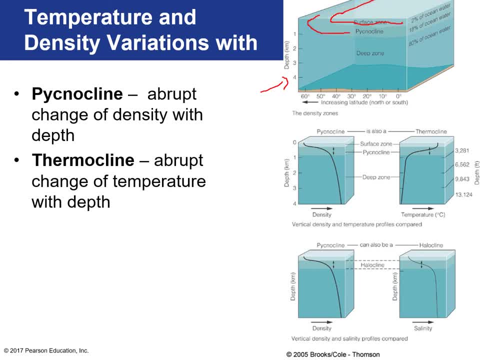 two percent of the ocean. then here's what we refer to as the halo Klein or peak. no, Klein makes up about 18 percent of the ocean. okay, that's where you see a drastic increase or decrease in salinity or a drastic increase in or decrease in temperature. then here's the deep zone. 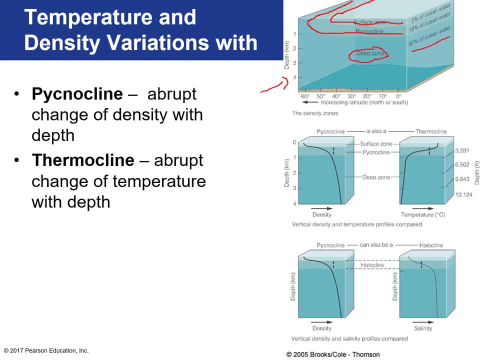 this makes up the majority of ocean water. okay, so the peak no Klein is an abrupt change of density or with depth, and that's basically the result of it is because of temperature. drastic changes in temperature in the ocean water leads to changes in density. okay, so here if we look at a cross section. 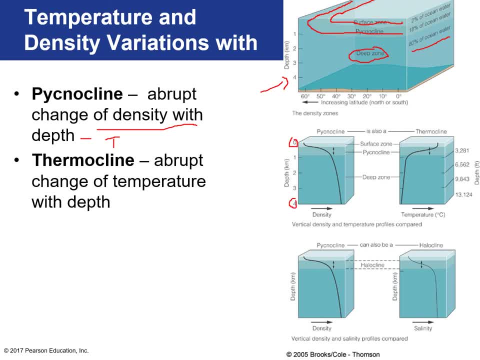 of ocean water from the surface to about four kilometers of depth. here's the surface zone and we'll look at temperature right. so here's temperature is fairly constant. for the first 100 there's a drastic decrease in temperature and temperature drops very rapidly. okay, so here's. 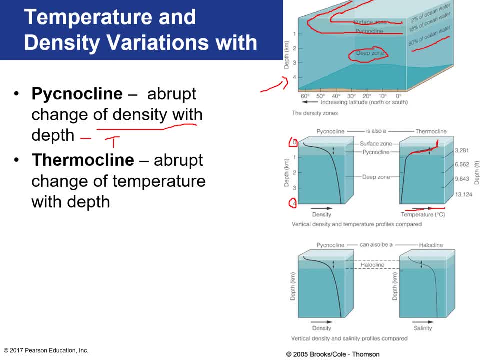 temperature. higher temperatures are over here, lower temperatures are in this direction. so what happens is if you were like, say, you were swimming in this water and you could somehow go deeper and deeper into the ocean water, it would get colder and colder, as it would remain constant for the 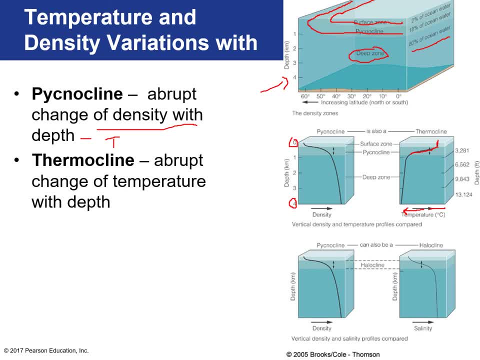 first, let's say, hundred meters, then once you go beyond that, then there's a drastic decrease in temperature and then once you get down to the deep zone, it kind of levels off, okay, and so that corresponds to changes in density. so higher densities over here, lower densities over here. so increasing density goes in this direction, okay. so 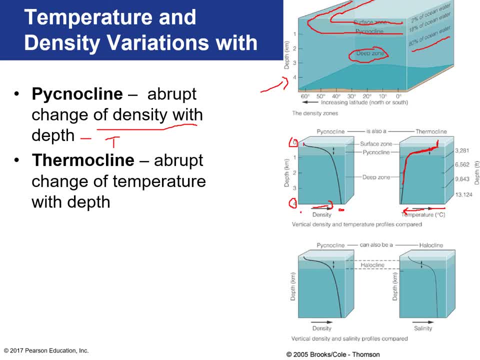 what happens is you have very low density water at the surface and that's because temperature is pretty high. but then the density drastically increases right here at the thermal Klein or peak- no Klein- and the reason why the density increases is because the temperature is dropping. so temperature drops means 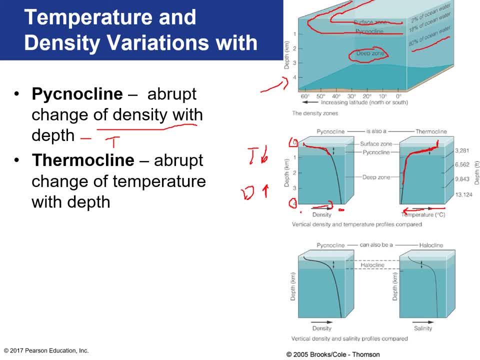 density goes up and so that makes a whole new mass of water right that sits on top of the deep zone and then as you go into deeper and deeper water, the density kind of levels off because the temperature also levels off. okay, and that's the same. it also holds true with the 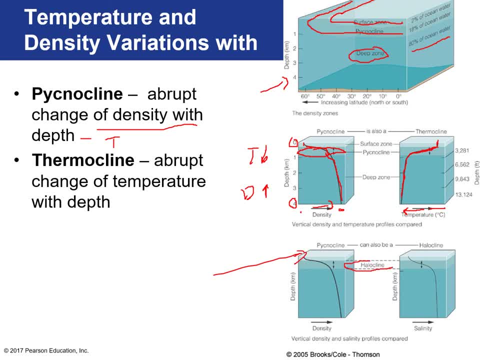 halo Klein. halo Klein is this area here, and that's where you have changes in salinity with ocean depth, and so essentially, what this does is this: segregates ocean water into different masses of water. low density ocean water will sit on top of the higher density ocean water. all right, here is temperature. 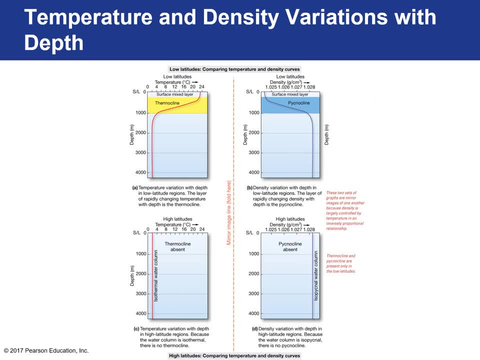 and density variations with depth based on two different latitudes. so over here are at low latitudes and this is at high latitudes. so at low latitudes, you know in the Caribbean, or you know on the coast of Colombia or Ecuador or something like that, you have really hot waters at the 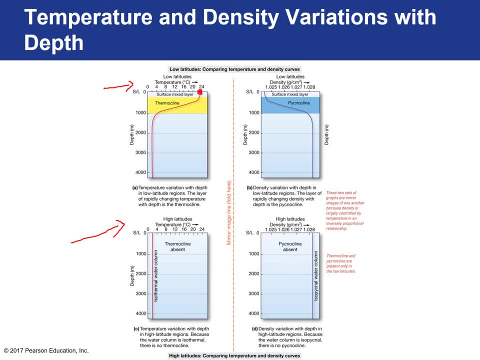 surface, surface mixed layers, really warm waters, but then once you go into deeper, deeper waters, it starts to temperature decreases rapidly, okay, and then here is the thermal Klein. this is this ocean layer here that goes down to a depth about one kilometer. the peak, no Klein is, is the kind of opposite, right. so the surface mix layer. 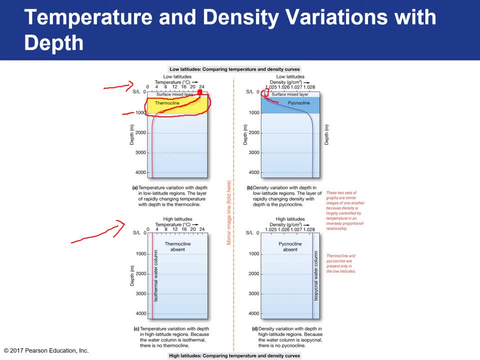 is very low density, but then density increases sharply in that same layer up until about one kilometer and then density kind of levels off and temperature levels off and it, you know, these temperatures is about like two degrees centigrade. so if you're in a submarine down two or three kilometers, 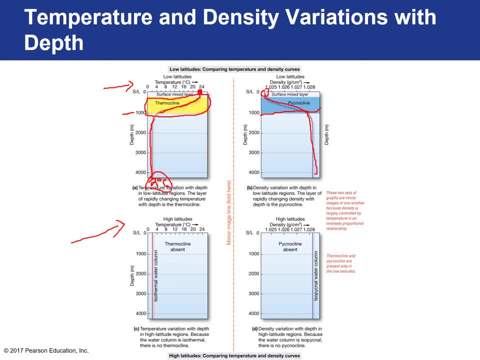 it's two degrees centigrade. that's very pretty cold, okay at high latitudes. so if you were up in like the Bering Sea, if you're in off the coast of Norway or something, there aren't these ocean layers, it's all the deep ocean, one one layer. there's no change in. 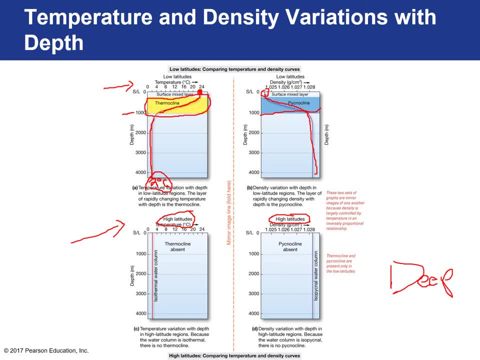 temperature or in density. these are called isothermal water column, meaning like if you're on a boat and you fall off into the water. here it's two degrees two to three degrees centigrade, and that temperature doesn't change whether you're four kilometers underneath the. 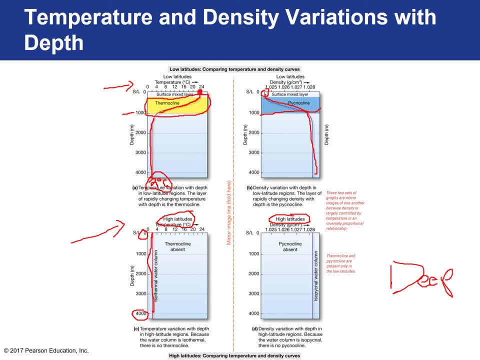 the ocean at a depth of four kilometers or you're on the surface, so the temperature is the same on the surface as it is four kilometers deep and we call there's. that means there's no thermocline at these high latitudes and also there wouldn't be any peak, no climb or change in density. the density of the 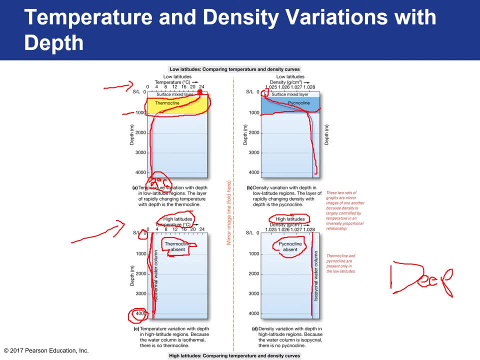 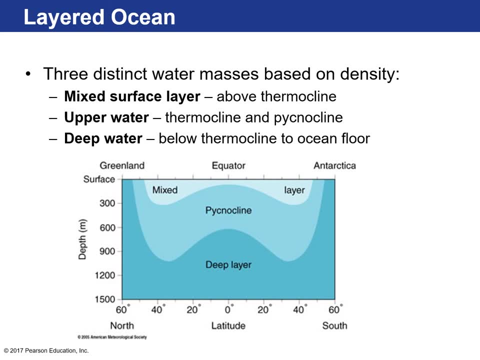 ocean water at the surface versus four kilometers of depth is the same. okay, so this is our layered ocean. we have a mixed surface layer that's above the thermocline. we have the upper water, which is the peak- no climb or thermocline, and then there's that deep water. so at high latitudes, this deep. 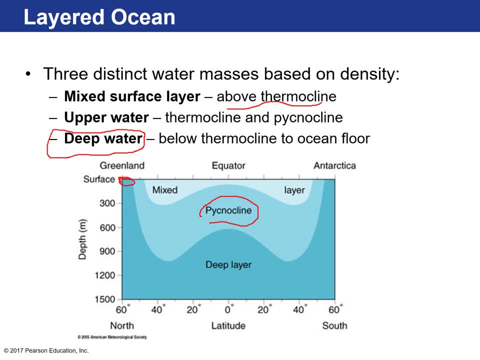 water, see that it's on the surface of the earth at the high latitudes in the North Pole and in the South Pole. that's why it's so dangerous to go. you know that the deadliest catch- I don't know if you ever watch that show, but those 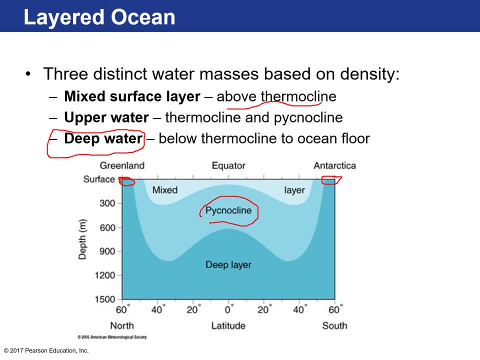 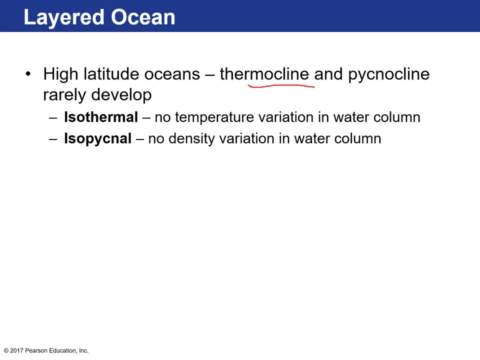 fishermen. if they fall into the water the get hypothermia pretty quick. so water is very cold. so at high latitudes those ocean layers- thermocline and peak no climb- really rarely develop and so we refer to them as isothermal or ice- I saw Nicole- where there's no density. 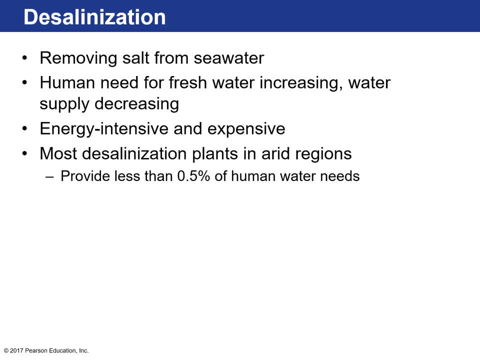 variation. okay, now let's talk about how. how is it? how is it possible to remove salt from ocean water? we call that desalinization. our needs for fresh water is always increasing because we use it for all kinds of purposes, but a lot of times it's very energy intensive and expensive. 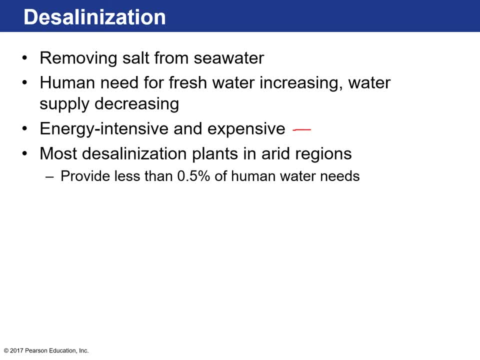 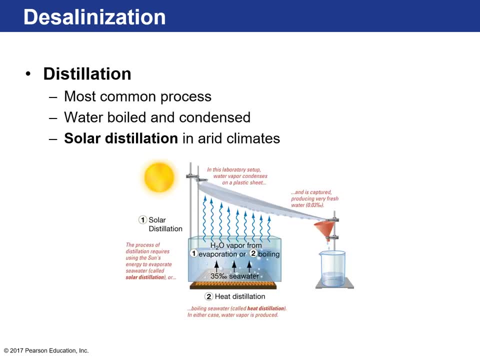 and so desalinization plants- really they only provide 0.5% of human water needs because they it costs a lot of electricity to kind of desalinize ocean water, the most common method. and this is a cool survival tool if you ever stranded out in like somewhere away from. 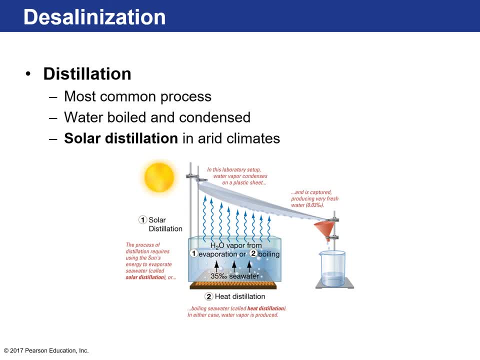 civilization, but it's called distillation. okay, this is the most common practice. when you, when water is boiled, or if ocean water evaporates, it can condense, and that condensed water is pure water and you can use that and you can drink it. solar distillation can be used in really arid climates, and so what? 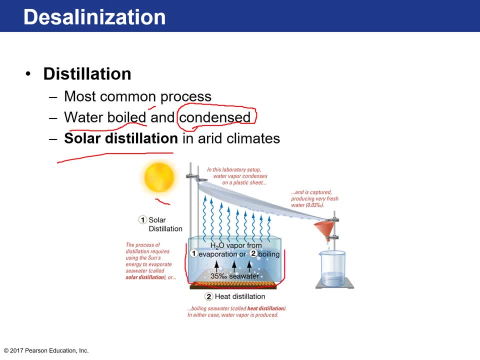 you do is you have a lot of water and you have a lot of water and you have a lot of ocean water in a container that gets heated up by the Sun. that water starts to evaporate, and then you drape some plastic over it and have it tilted. 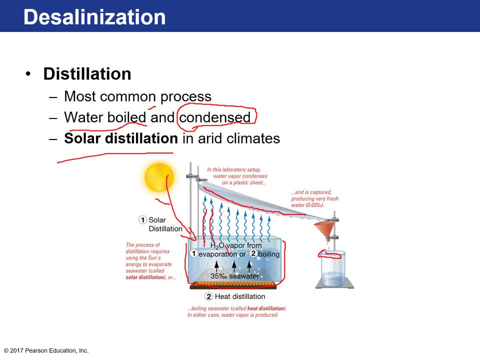 towards a beaker and a funnel and all that evaporated water will be caught by this plastic sheet and under the force of gravity will condense and then move down in this direction and then drip into your beaker. very slow process but this can be done, kind of like an 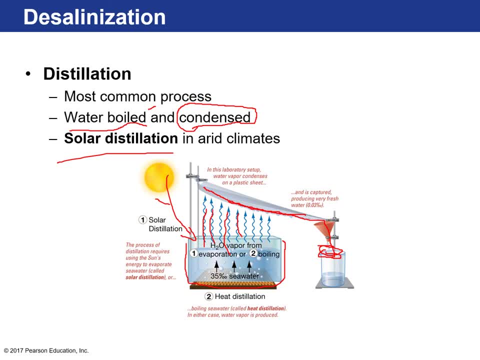 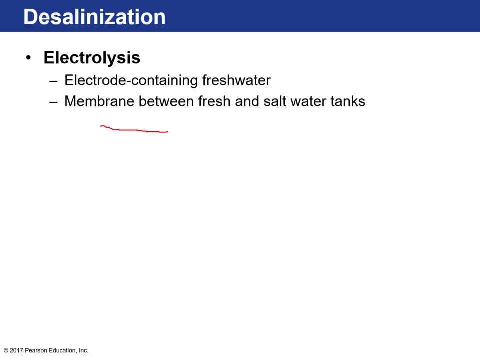 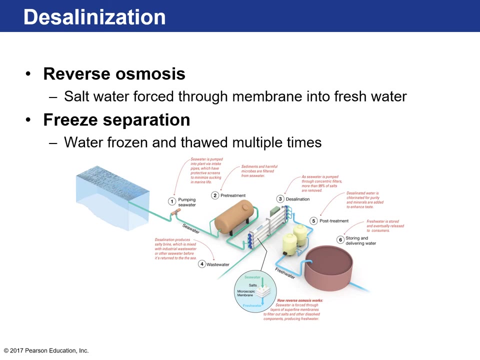 makeshift way if you're ever stranded, and it can help you survive actually. so then there's a electrolysis. this is where a membrane is between fresh and saltwater tanks and you help pass it through. here's an example. you pump seawater through. here. there's some pretreatment. here's the desalinization. 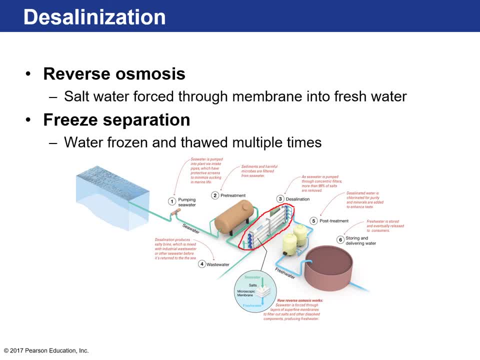 running through those filters removes about 99% of the salts itself, and then here's the storage and delivery of that water. So that's a more complicated process and it's very cost-intensive. Then there's freeze separation, but that's probably more efficient in cooler areas. But when you freeze water and 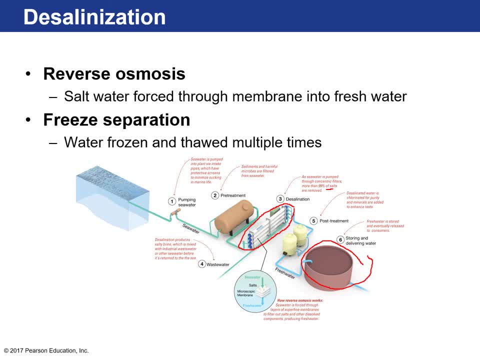 thaw it like say you freeze it, only fresh water will be frozen and then you can thaw it later and actually drink that water.